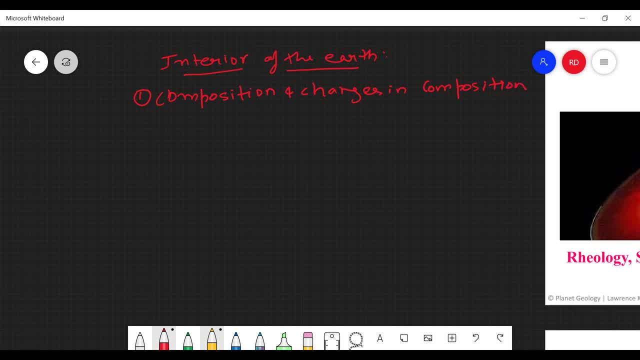 Okay, and the second thing that that we want to understand is are the mechanical properties. mechanical properties and what other thing? mechanical properties and rheology? Okay, rheology relates to the flow, more or less, and mechanical properties And rheology. So say same composition doesn't mean that they will have same mechanical properties. For example, iron, when it, when it is cold, it behaves differently. When iron is red hot, it behaves differently. When it's molten, it behaves differently. So the same composition can have, or say same composition material can have different properties. Okay, so these are the two main things that we want to understand. Okay, we want to understand the changes And when we are talking about structure, we want to understand the changes. 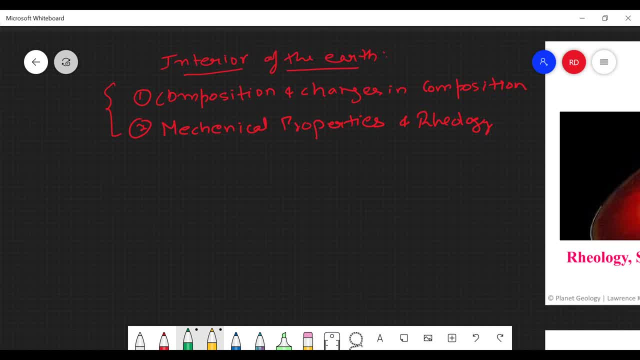 And when we are talking about structure, we also need to have an idea of at what depth those changes are happening. Okay, so you also need an idea about the depth of those changes. Okay, And because we'll be measuring these properties. so there are different ways in which we can actually know about the interior of the earth. how do we know what is present inside the earth? but there are two main, two main things that we want to understand. Okay, 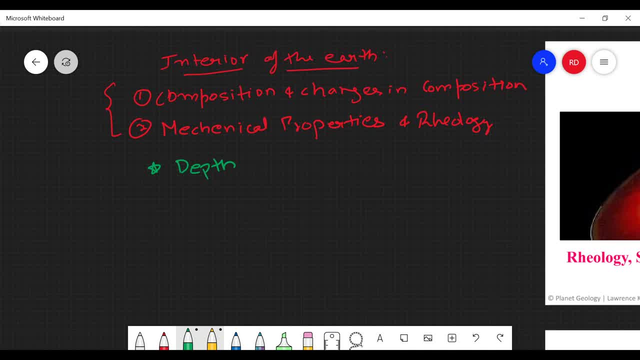 So can you tell me what are, what evidences can we use or what sort of physics can we employ to understand the interior of the earth? Okay, So what are the tools? tools for us to understand the interior of the earth? Seismology. 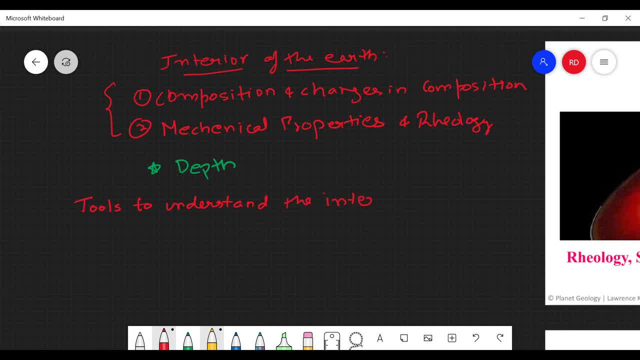 Understand the interior of the earth, Okay, Yes, someone mentioned study of seismic waves. seismology ampl. exacerbs好不好, Okay. Okay, Those who are not from geology background, seismology is a study of basically seismic waves, how they respond when they travel through rocks. Okay, so what are seismic waves, you may ask. seismic waves are just like kind of acoustic. 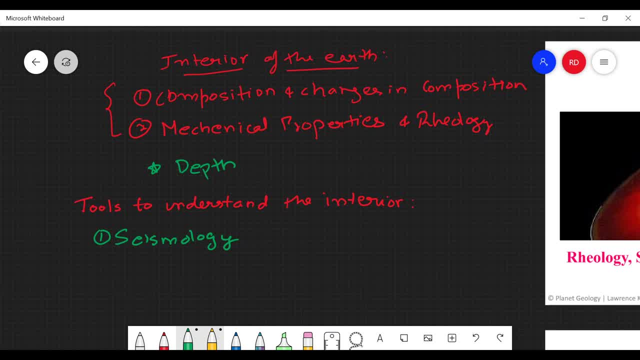 waves which Travels Through the surface of Earth. they are. they're generated in some manner. they could be natural or they could be man-made as well. Now you may ask: what are acoustic waves? Okay, waves are just type of mechanical waves, for example. if i'm speaking right now, so my voice 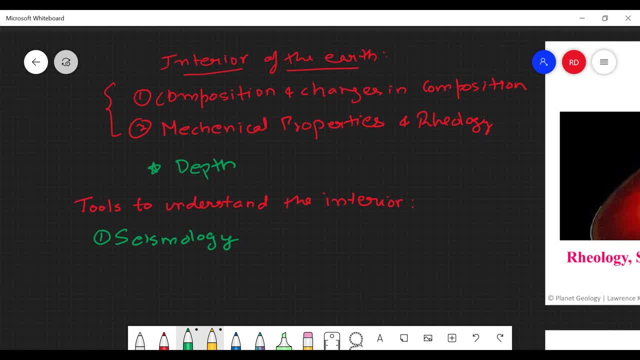 is is a kind of acoustic with the sound wave, is a kind of acoustic wave which has which are which are caused by vibrations of actual material, okay. in contrast, for example, when you look at light, light is also a wave, but it is an electromagnetic wave, okay. so here the material itself is not. 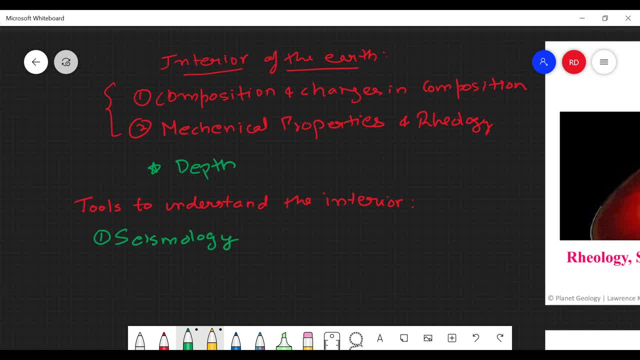 vibrating. it is rather vibrating electric and magnetic fields. electromagnetic waves do not need a medium to travel. acoustic waves need a medium to travel. okay, so sound waves are other type of acoustic waves. if you hit you the surface with hammer, or even with your feet if you're dancing, the floor starts to vibrate. those are also types of seismic waves, only there. 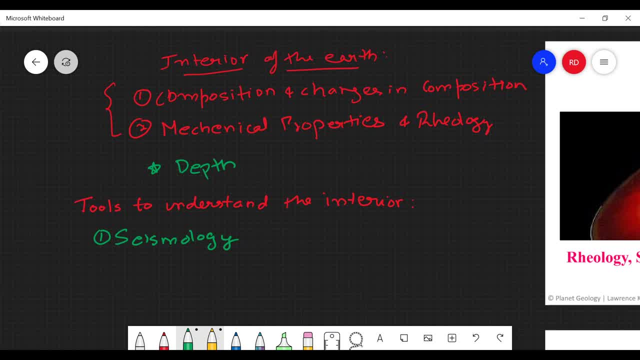 is there no way different from the seismic waves you're talking about? what tells about earth we actually need? because if you want to know the internal structure of earth all the way to the core, all across the earth, we need a very strong source of seismic waves. okay, so that source is usually what we call. 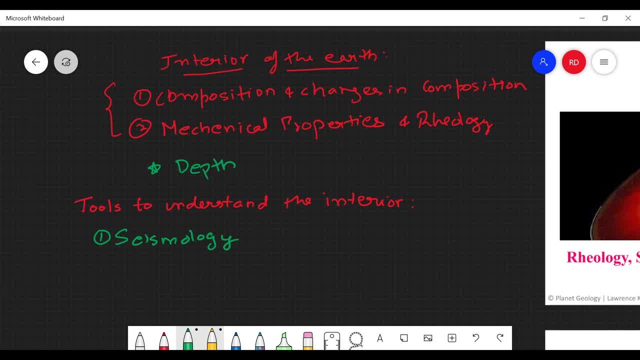 earthquakes. okay, so earthquakes are a source of seismic waves- that is what you feel when the ground is shaking- a type of seismic wave. okay, and those seismic waves, they travel inside the earth and, based on these changes in in velocity, they are refracted, they are reflected of different discontinuities. so that is what can tell us about the internal structure of 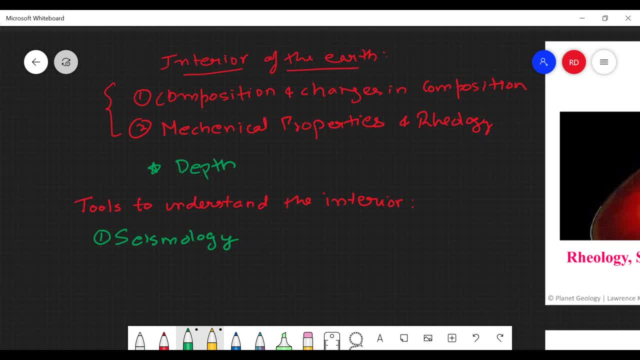 the earth, of the earth under the seismology. so that is the main. this is the main most important for us: to understand the internal structure of the earth'. what else can, can we use, for example, if you want to know what could be the bulk composition of the earth, what, what? 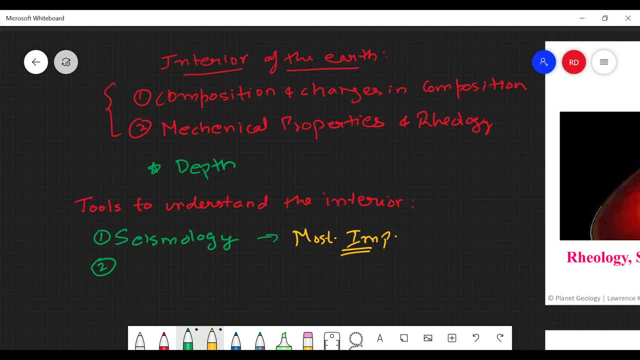 other tool can we use? we studied one yesterday: meteorite meteorite. yes, about meteorites. think someone mentioned ophiolites. i'm not sure if i heard it correct, but ophiolites were still pretty shallow level, like okay, you're still in the crust, only maybe a little bit of little bit. 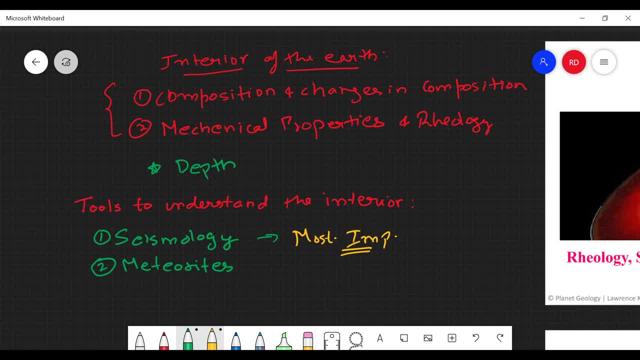 of like there's just the lower part of the crust where there is, like, some ventils. you know let's, but it's, it's most importantly if you want to know meteorites, because they tell you about the composition. because if you look at meteorites, for example, if the amount of iron in meteorites 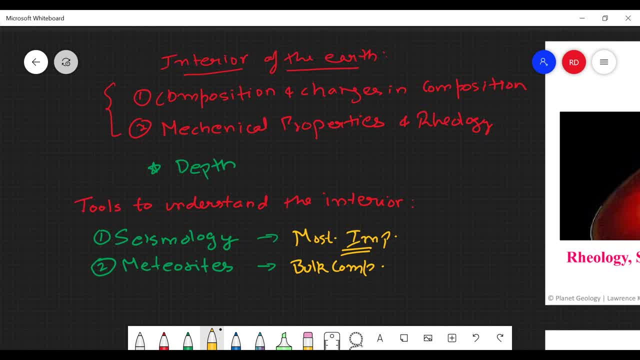 is much more than the amount of iron in the crust or the mantle. so that tells about that there should be somewhere more iron source in the earth. some of the meteorites are made of pure iron, so meteorites also tell us about the internal structure of the earth, or rather they act as like any models that 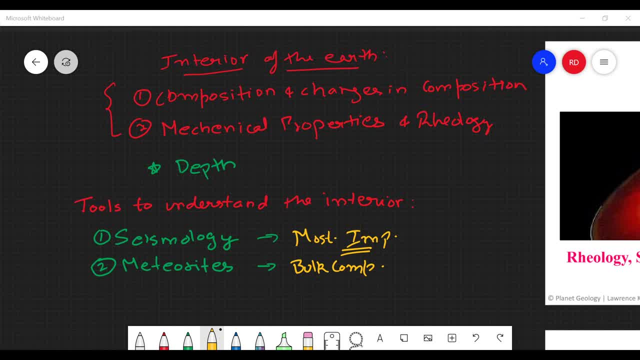 we build about the internal structure of the earth, they will act as constraints. okay, so whatever model i we build, you say, okay, the composition should match this particular value, and i've derived that from the meteorites. what, what other features do you think we can have? you see, it's it's easier for us to know about surface of mars than it is to. 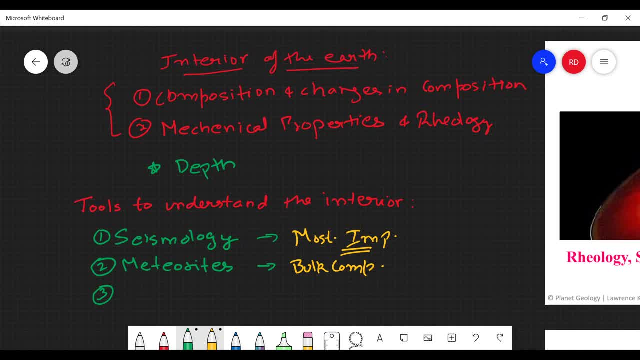 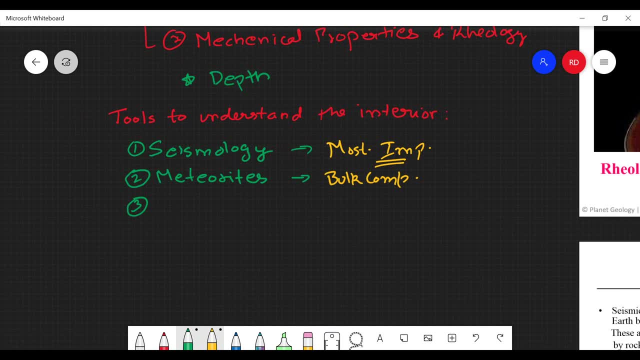 know about the interior of earth, what, what else can we know? the structure of rocks, structure of rocks, okay, or simple what, what we'll call it lab experiments. a structure of rocks also will come. so how do rocks behave? so, as you say rocks, so how do rocks? 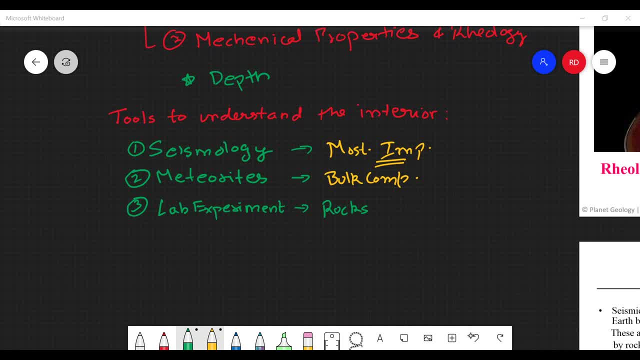 behave? how will rocks behave under due to changes in pressure, temperature and stress? okay, rock behavior due to pressure: okay, temperature and stress changes. now, for example, you have a particular type of rock on the surface- okay, or, or you may make it also based based on, like, some rocks which you have recovered. you can think like you, you can do. 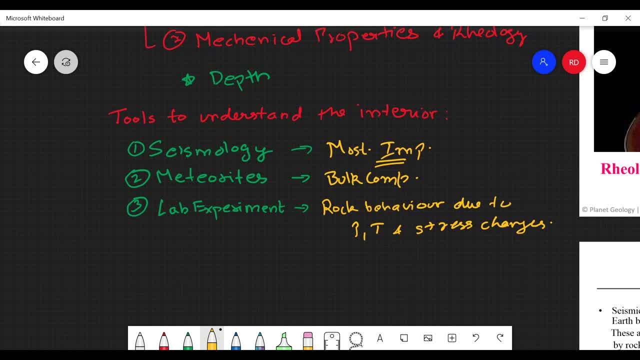 experiments. if i increase the pressure, you cannot go below, for example, let's say, to the core mantle boundary. but what you can do is you can try to recreate the pressure and you can do experiments as best as you can. some of those conditions you can subject rocks or minerals. 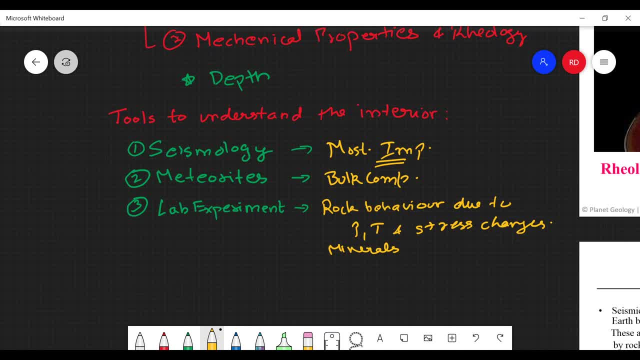 you not just like rock, you can also call it minerals. to high pressure, high temperature, let's say stress also: how do they behave? do they behave in a ductile manner or do? are they still brittle? so all those experiments you can do and that that will give you an idea of what one those minerals won't be there, what if there will be any phase changes, and all of just that cover process that you can do and that that will give you to get the ideas like how 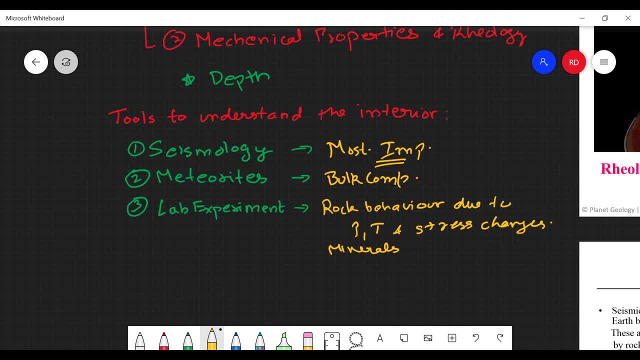 health of minerals stay the same, which is sh기가, grouped, floating and meaning all all things like that. anything else, what? what else can we use? yes, yes, yes, you can do about xenoliths. what else? volcanoes again, that that that will be part again come under xenoliths only. 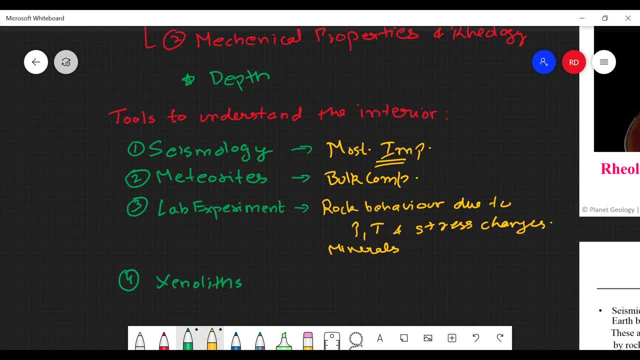 okay, let me. let me call because volcanoes, if it is crustal material melting. so again, these are for like slightly shallow levels. okay, let me call it volcanoes. okay, anyway, volcanic rocks are present on the surface also. okay, so they tell us about a little bit about the uh, about the internal structure. let me write ophiolites also here, those who do not. 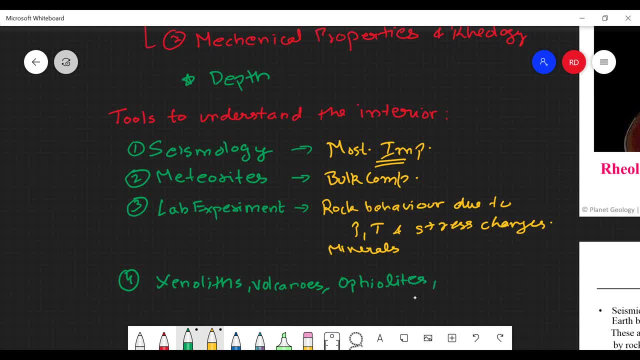 understand ophiolites. don't worry, we will come to this particular part. for the time being, it's just oceanic crust which is abductive onto continental crust, but we'll come to this part. xenoliths, volcanoes, ophiolites- i'll cover or complete all this in this particular part only. okay. 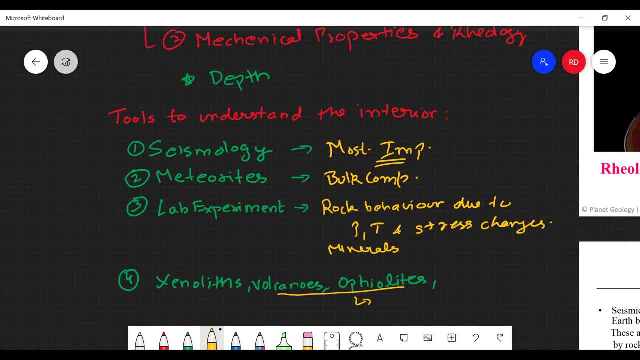 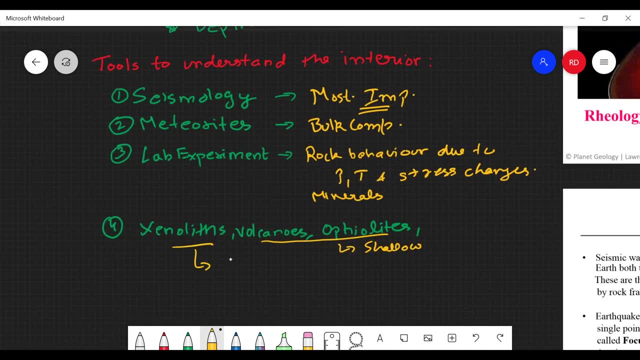 so, but again, these, these especially, will tell us a little bit about shallow level. okay, this xenoliths, again, intermediate, yes, any, any, any other study of mental, study of mantle plumes, exactly again, see, the problem over there is: how do you know they are mental plumes? okay, until you know the something about the mantle itself, okay, how would you know? 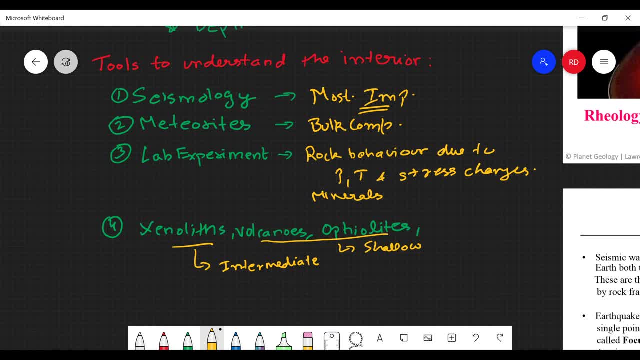 that they are mental plumes. so it's it's like you: you need to know one thing before other hand. okay, so we, we already have some idea about that. these plumes are coming from the mantle. that is how we know. but anyway, i will write it because if we know it from some other resources, then that can. 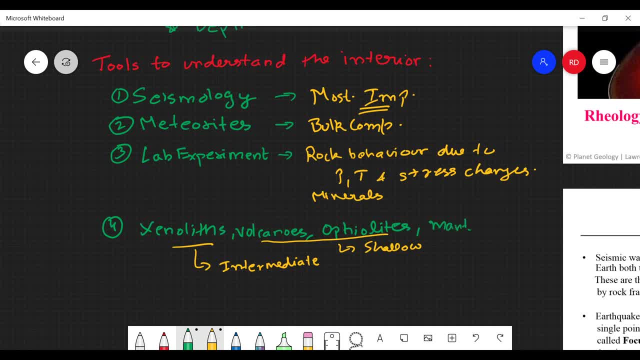 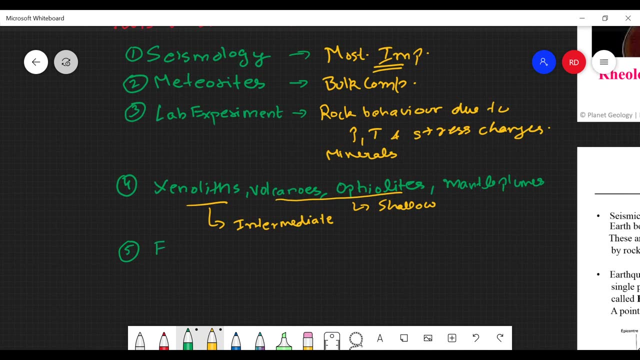 help us about it. okay, mantle plumes, you can study these. okay, but none of these will tell you actually about the core itself. okay, so then there are other evidences, use evidences such as earth's magnetic field that provides some constraints. okay, so you need to have something inside the earth that gives rise to. 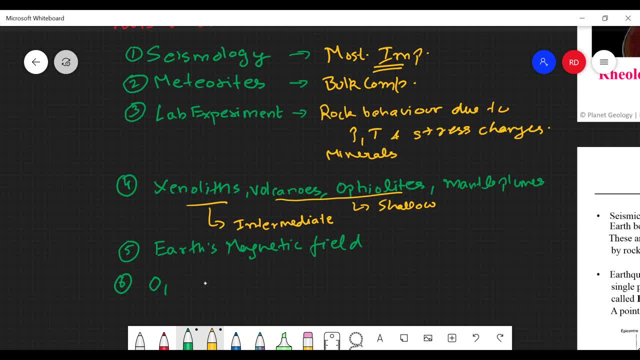 magnetic field, you can observe other planets. okay, observe other planets. why? because earth you can see only in given time. but if you look into the universe, okay, you will see planets in different stages of their formation, even solar, for example. we were talking about, uh, that, that proto-planetary disc? okay, solar, never. 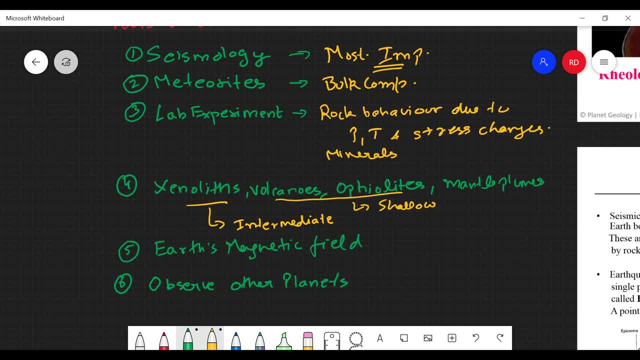 happened. but if you observe other planets in the universe, you can actually see those in the sky today because they are in different stages. okay, observe our other planets in universe in different stages, which are in different stages, so this tells you more about like how, again tells you about the 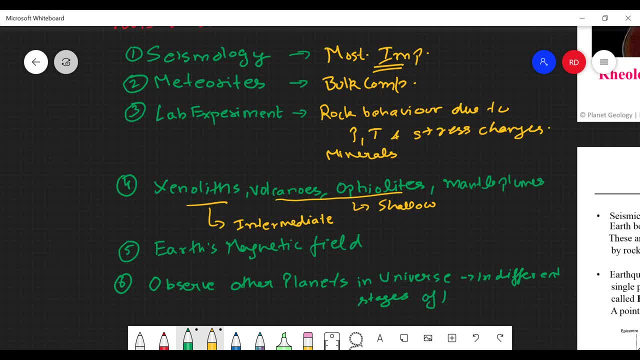 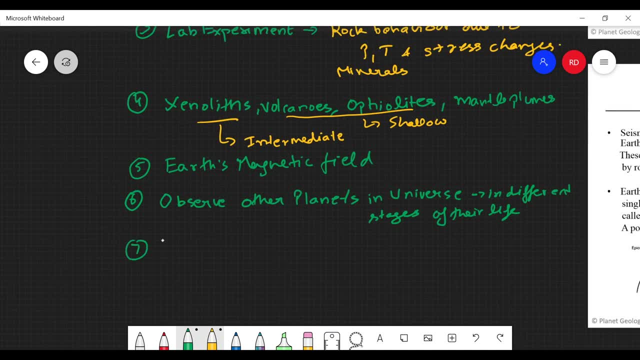 physics, what, what could have happened, and that tells us. so you, about the structure, different stages of their life. okay, most important one, we have already forgotten, and that is mathematical calculations. okay, for example, you need to know about you, you can calculate mass of the earth. okay, you can observe the rotational period of the moon. there are many. 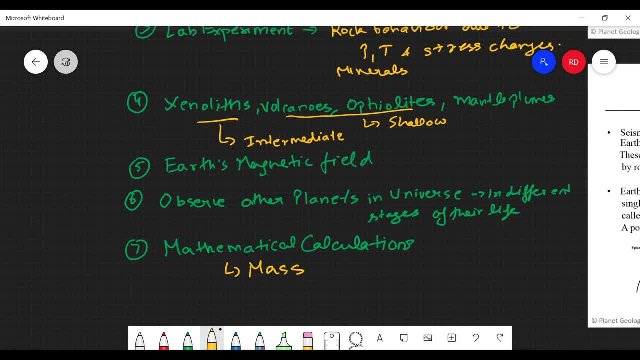 indirect ways to calculate mass. so you can calculate mass, so mass must match, okay, so what is the mass of the earth? so you, whatever internal structure you propose, for example, instead of iron co in the core, if you put gold over there, earth will become much heavier. so 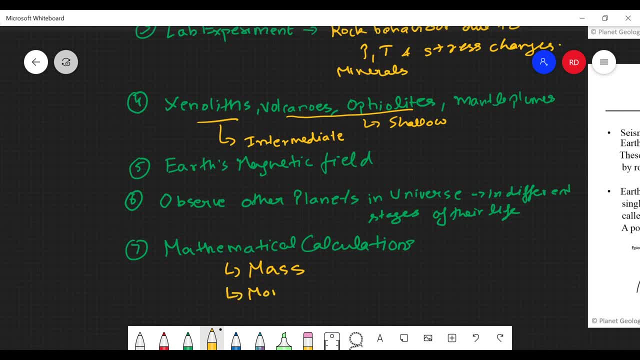 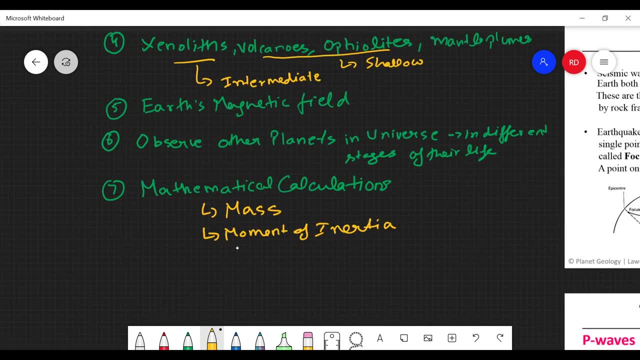 you cannot have that. other things such as moment of inertia, okay, etc. etc. so these constraints should also be met. some mathematical calculations to match all these properties. so there are actually many different ways to to learn about the internal server you you already talked about, uh, seismic waves. i will just in its point right in general geophys. 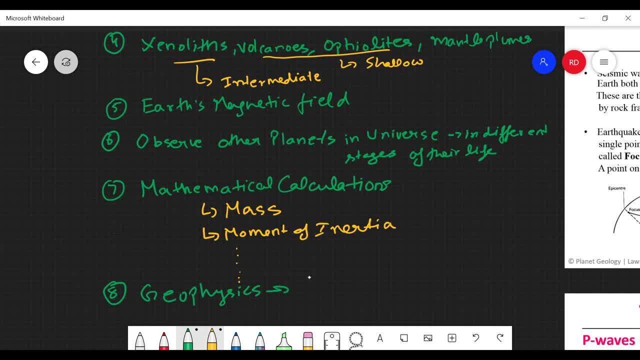 earth's magnetic field will also come inside geophysics, part only. but for example, magnetic tellurics, okay, electromagnetic surveys and all all these can, can also, all the electromagnetic surveys will be more useful in the shallow levels. but magnetic tellurics, for example, some, some of those can be, uh, used to understand the deeper structure. okay, so again, these, these. 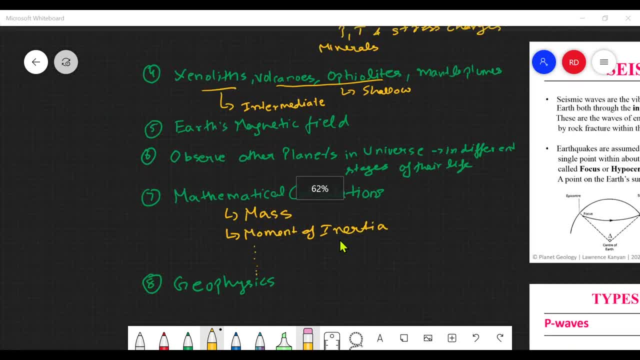 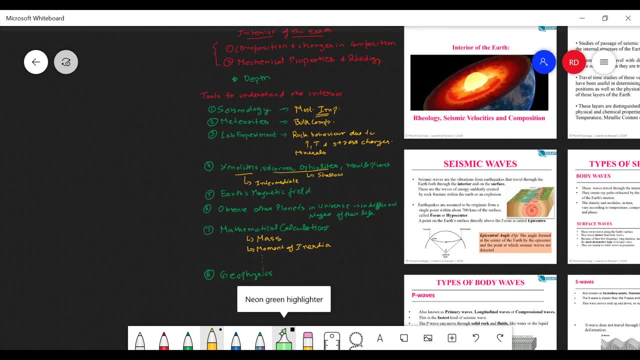 are some of the ways in which we we can learn about the internal structure of the earth, the most important. but which of these is the most important, sir? uh, timber light can be also tool. yes, again, you think of it. is is like part into coming into xenoliths, where where you get like you can study stuff from, from. 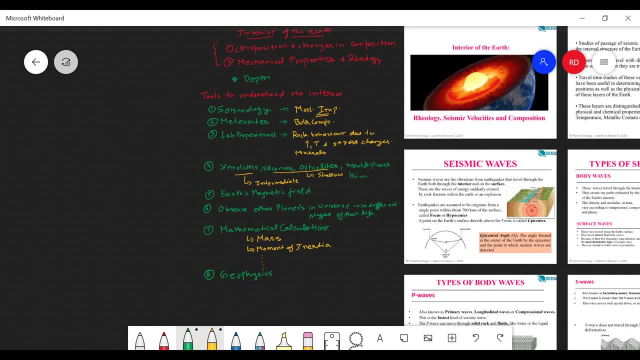 the deep parts of the earth. okay, i'll write it. kimberlites and all all this, etc. okay, all this will come. come here. uh, those who do not understand a few of these terms, don't worry, we'll come to kimberlites and all later on in in the subsequent lectures. you don't need to. 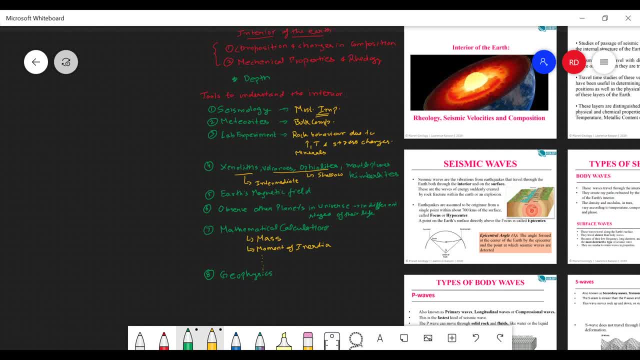 know them right now. but this, this is overall part- the most important that we will study is: what is the study of seismic waves? okay, we need to know a little bit about this particular part. okay, and that is what we will focus on. we will try to understand what seismic waves are. what are? 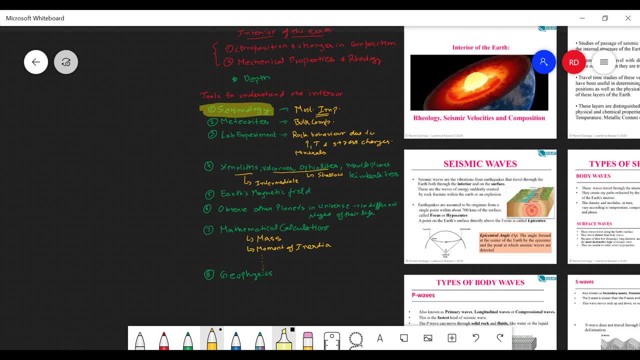 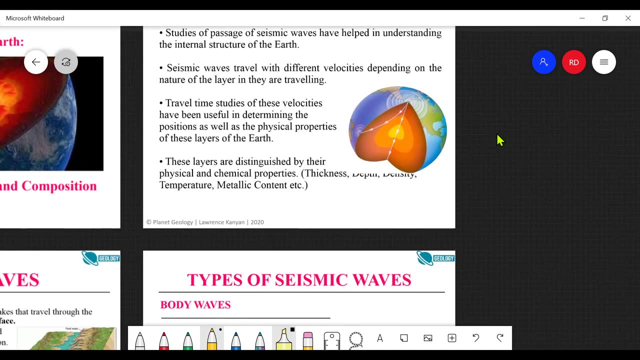 different types of seismic waves. for example, one question that you get very frequently is is just to write about types of seismic waves. okay, p waves as well, all this. so this: this question is pretty common for the upsc, uh, civil services exam. okay, so we will start with the slides now. you already 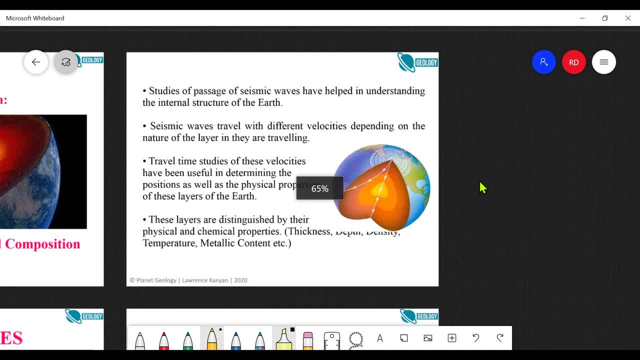 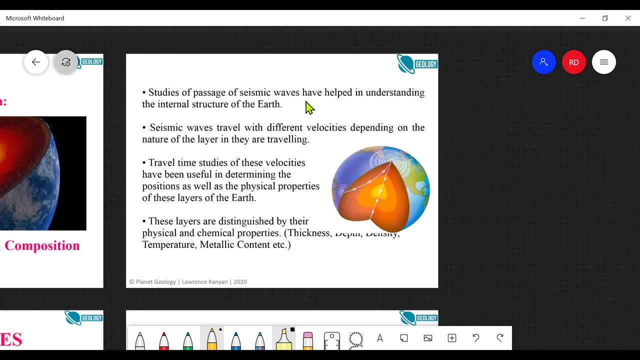 understand if you think of of some other terms. of course there can be other evidences as well, okay, about the internal structure of the earth. so studies of passage of seismic waves, let's say here: what is shown in this figure is: is that earthquake is generated pretty close to the surface. okay, 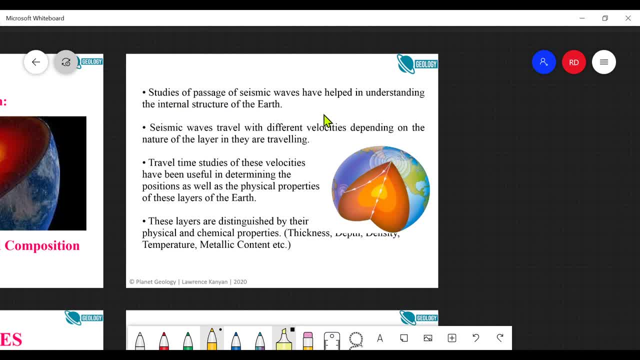 so within the crystal part in here. so studies of passage of seismic waves have helped in understanding the internal structure of the earth. the important thing is seismic waves travel with different velocities depending on the nature of layers in which they are traveling. okay, this change in velocity will will cause what is called refraction. just like with light, you have refraction. 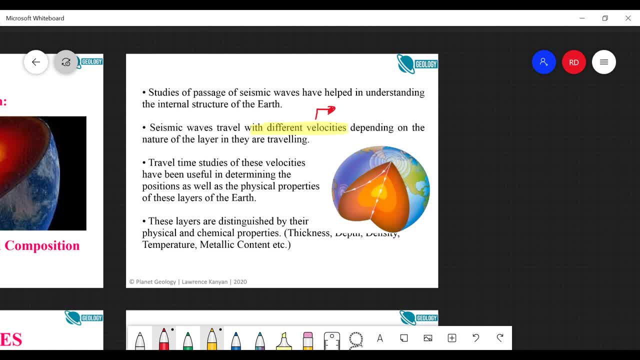 but when light passes- let's say it is coming from air or vacuum- and it goes into glass, it gets refracted. and the reason it gets refracted is because the velocity of light in vacuum or in air is more than the velocity of light, the velocity of light inside the glass. okay, so change in velocity results in refraction. 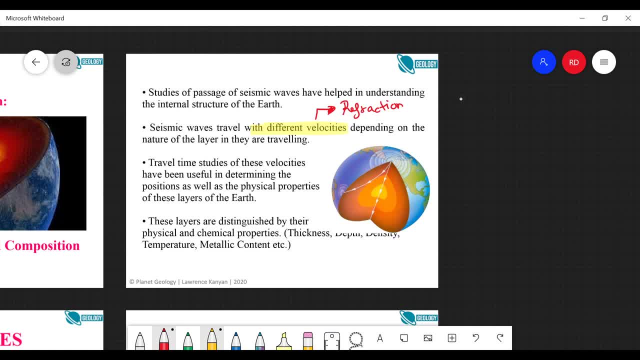 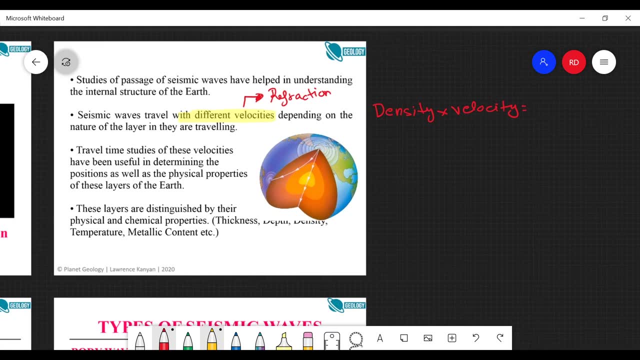 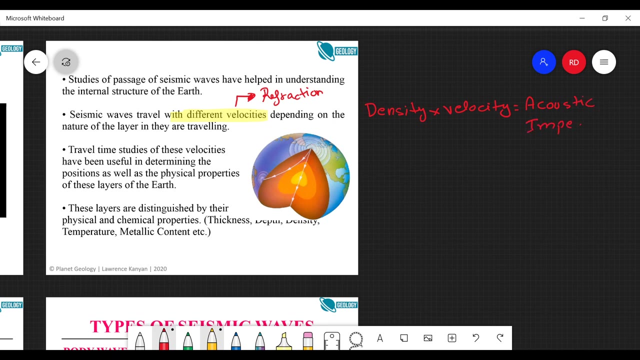 okay, and also we have a property in seismic waves in which you multiply density of rocks with velocity. okay, which is called. the product is called acoustic impedance. okay, this product is known as acoustic impedance. what does it determine? it will determine the. what does acoustic impedance determine? two determine: 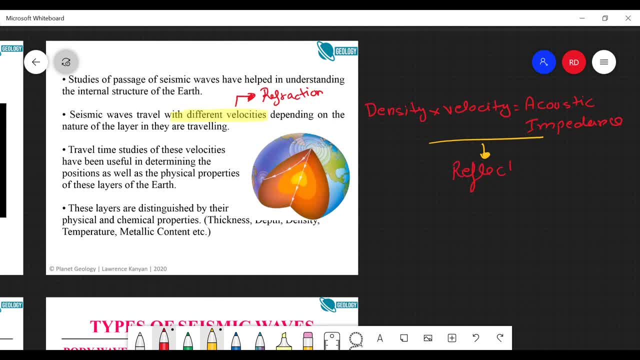 just like the waves get refracted, it will determine reflection if acoustic impedance from between two layers is high. so the product of density and velocity is called acoustic impedance of these seismic waves in a, in a rock. okay, that is what we are talking about, so that will give. 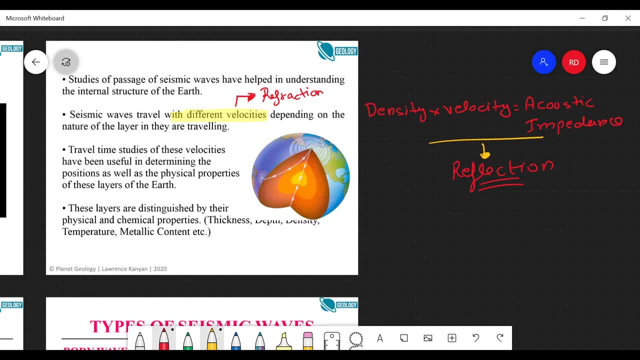 result in reflection. if there is high acoustic impedance contrast, so the acoustic impedance of one layer is very different from that of other layer, it will result in reflection. the stronger the acoustic impedance contrast, the stronger will be the reflection. okay, so these reflected waves come back. so it's kind of like an ultrasound that you do. okay, so you can see how much time does it? 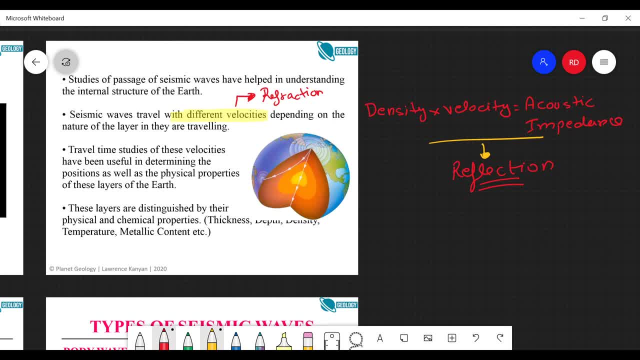 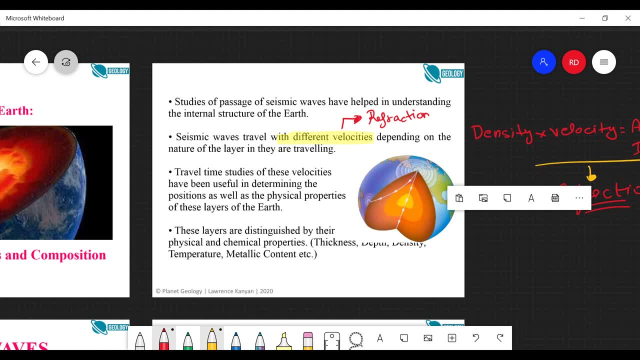 take for the, for the waves to reflect back, and then you can study the, the reflected waves. in reflection seismology. you can study the refracted rays and that will tell you about the internal structure of the earth. so travel time studies of these velocities have been useful in determining 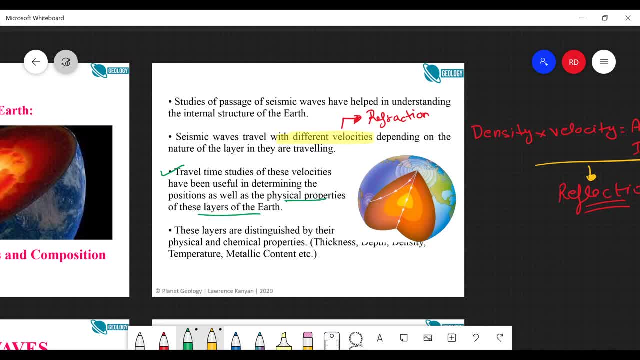 the positions, as well as physical properties of these layers of the earth. okay, so these layers are distinguished by their physical and chemical properties. so that is what we are saying: physical, mechanical properties, rheology and the composition and the things that that we also need to be to to. that we need to understand is the thickness, depth, at what depth, those discontinuities. 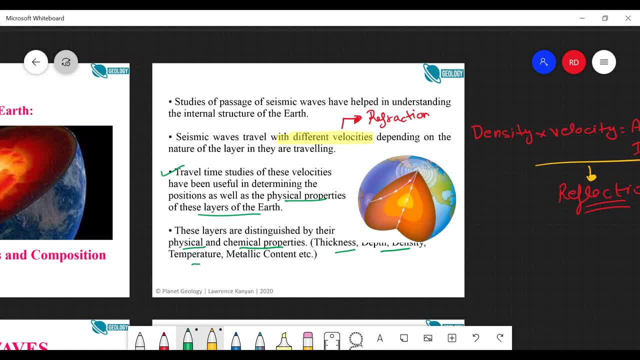 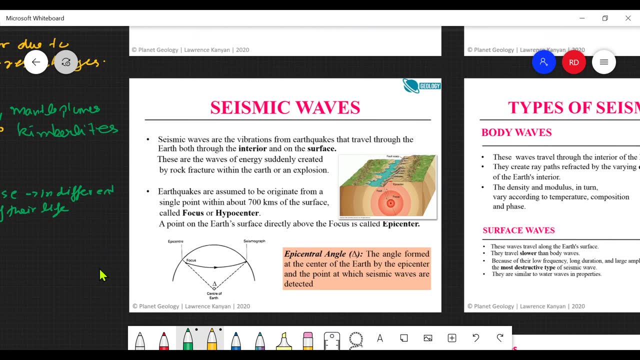 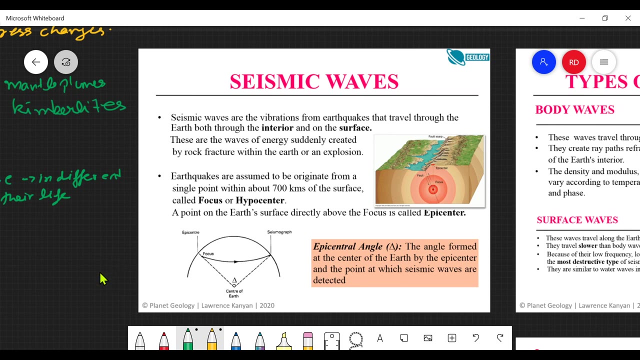 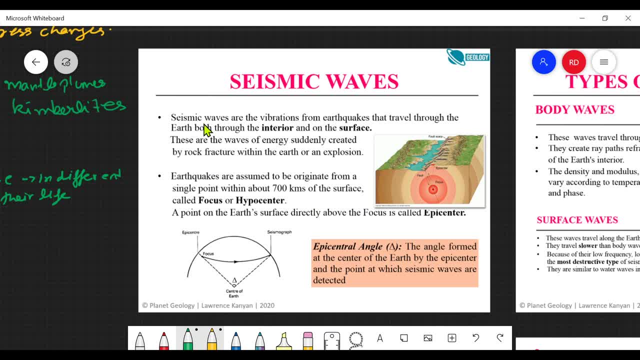 seismic waves all across the earth. so seismic waves are vibrations from earthquakes. so we are here talking about natural seismic waves. because they are strong, they can travel all across the earth. so these are vibrations from earthquakes that travel through earth, both through the interior and on the surface. okay, so they travel through the interior of the earth as well as they will travel through the surface. these are suddenly created by rock fracture within the earth or an explosion. 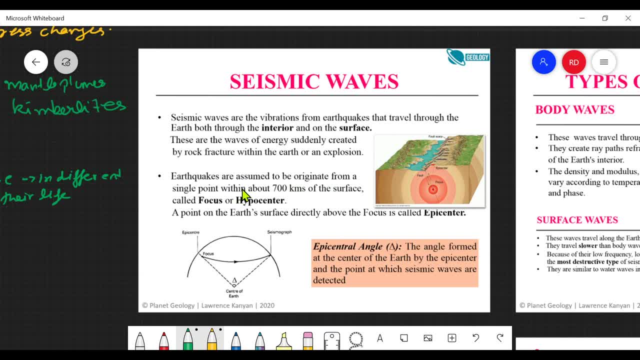 again, earthquakes are assumed to originate from a single point within about 700 kilometers of the surface. again, 700 kilometers is pretty deep, but you will never find earthquakes below 700. okay, usually you will find it within first few tens of kilometers. okay, 40, 50, 60 kilometer, not deeper than that. in some, some cases near plate boundaries, they go even deeper. okay, so, for example, in subduction zones- we will talk about what subduction zones are. 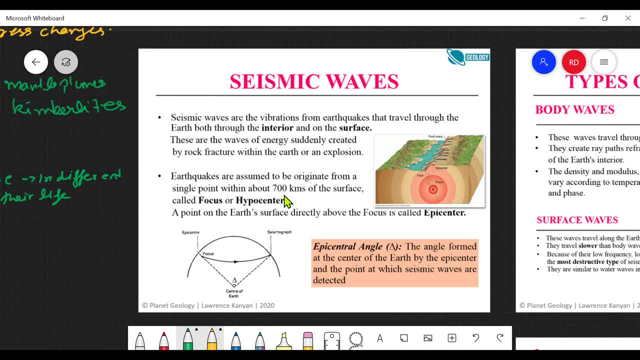 but usually they they are pretty shallow. they don't even go to this level, 700 kilometers. okay, only in special areas, special circumstances you will find earthquakes as deep as 700 kilometers, a point on earth surface, directly above the focus. for first, first example, we'll try to see what. what focus is the actual point at which earthquake occurs. okay, so this particular point, for example, is the focus. 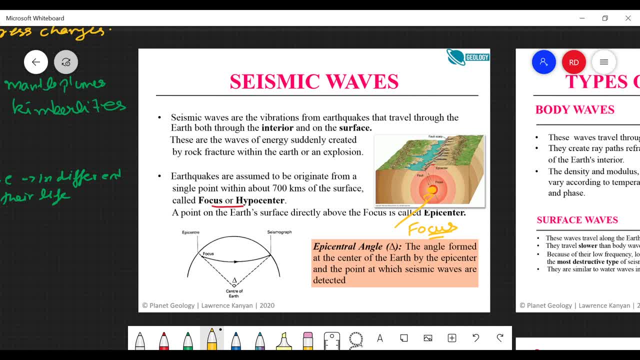 okay, so this is the focus, the actual angle and the point directly above the focus. okay, on the surface. so epicenter is present on the surface. so the point directly above the focus. it is called the- what is the name for that? so you have this focus here. it is the point at which earthquake is occurring. so, above the focus. you will have epicenter. okay, so epicenter is the point directly above the focus on the surface. so epicenter is the point directly above the focus on the surface. so the point directly above the focus on the surface. so the point directly above the focus on the surface. so the point directly above the focus. it is called the- what is the name for that? so you have this focus here. it is the point at which earthquake is occurring. so, above the focus, you will have epicenter. 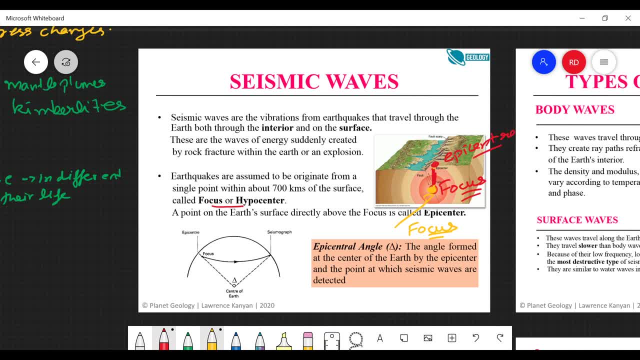 okay, so epicenter is present on the surface of the earth. so if you're standing on the epicenter, you can think of it that the earthquake happened somewhere directly under your feet at some some depth. okay, so if you going, if you go vertically from the epicenter, you will arrive at. 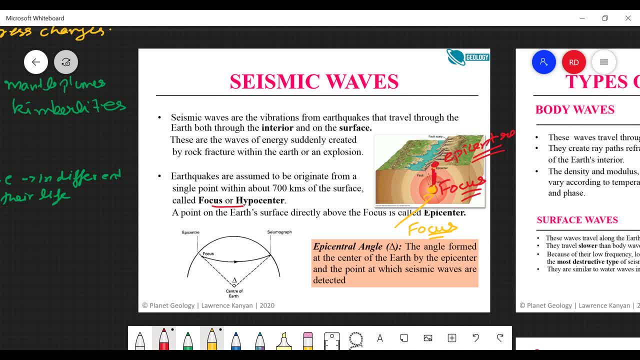 the focus. okay, now one thing. so there is. there's another term, which is epicentral angle. okay, again, not very important, it is the angle formed at the center of the earth. again, it is formed at the center of the earth by the epicenter and the point at which seismic waves are detected. okay, you will detect these seismic waves at some receivers by seismographs. okay, so you will have a seismograph which will detect these seismic waves and you can have it in different locations. so the angle between the epicenter and the seismograph, it can vary from different places. that angle is known as the epicentral angle. any questions until the end of the session. thank you very much for your attention and we will see you in the next session. bye, bye. 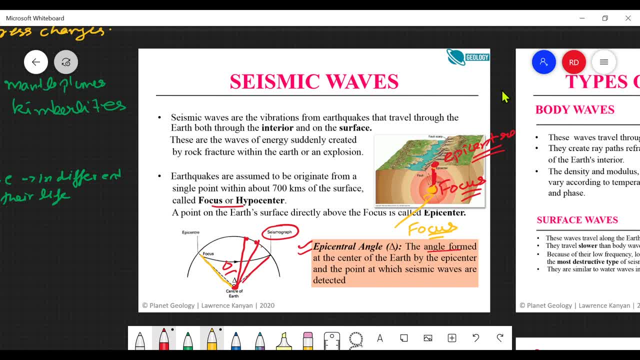 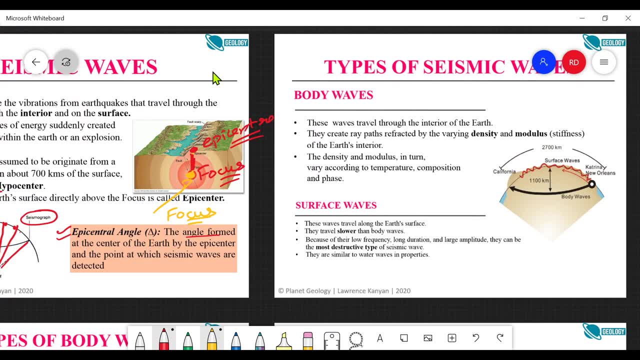 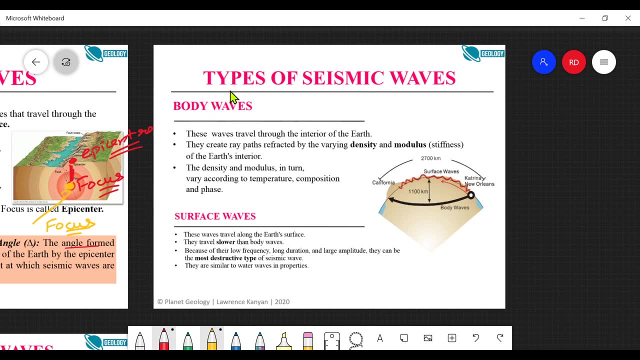 now, okay, now moving on to the different types of waves that we have. okay, different types of seismic waves which will be important for us. so, first of all, the most important is, like, body waves. okay, so what are body waves? so these waves? first of all, they travel through the interior of the earth. that is why they are known as body waves, so they 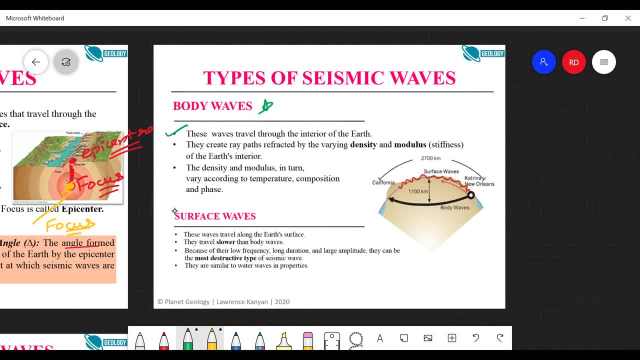 travel through the body of the material. in contrast, there is another type, which is surface waves. so they's not. they do not travel to deeper levels. okay, it's not that they are just on the surface, but they die. excuse me, sir, there is any source by which we can predict earthquake? right now there is no source by which you can directly predict earthquake when it is going to happen, but what. it is no source which way we can predict earthquake. right now there is source by which you can directly predict earthquake when it is going to happen, but what it currently name. but that will depend. so, as soon as front, let us predict that one of the last universe' Chinese rock convalescent Happy signified because its 없어요, it hasn't yet been thought about for its already present 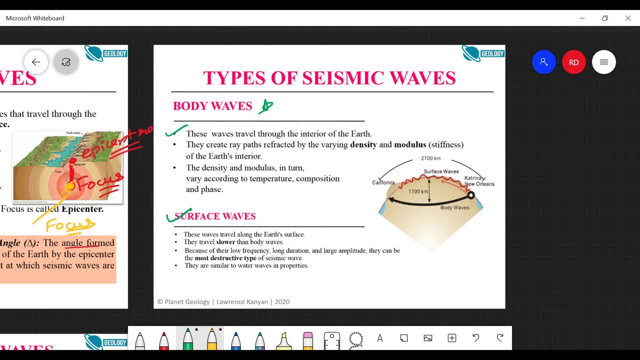 it means, like what you mean by predictions. okay, we have pretty much good idea where earthquakes occur. okay, so, for example, along ring of fire, they're very common earthquakes along subduction zones, so we know in which regions earthquake occurs. we can have an idea about probability of an earthquake occurring. okay, in this zone, there is high probability of an earthquake occurring. 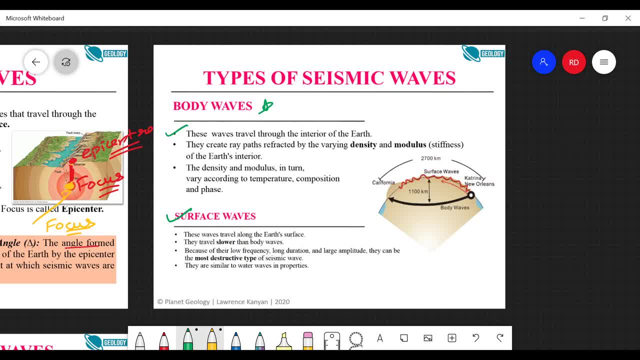 so it's not that we are clueless, we have some idea about it. that's why we have seismic zones in india. we'll study that part also. but if you want to ask, like when a particular earthquake will occur in a given location, about the timing, we still don't have any any any way to do that, okay. 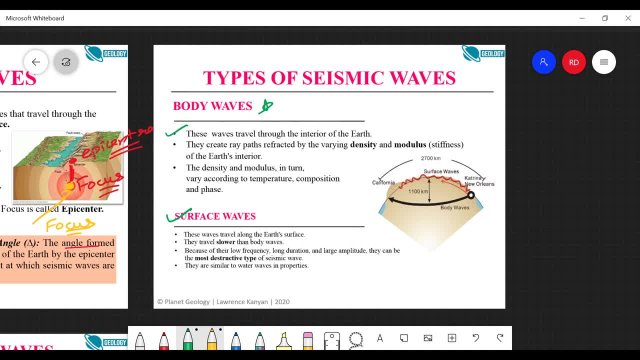 so, either way, don't say, like it's, it's completely random, it's also not completely random, okay. for example, we saw one earthquake in assam very recently. that was expected. i won't say that was expected, but we see earthquakes in that region. we expect that earthquakes will occur. 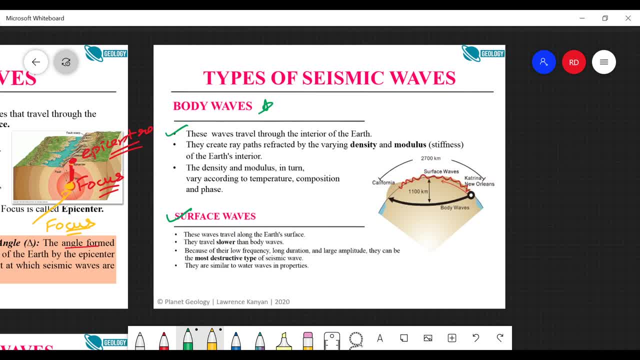 in the future also, they will not stop. okay, all right. so yes, so we're talking about body waves and surface waves. so we already know. body waves: they travel all the way through the interior of the of earth- or, yeah, in this case we'll talk about earth or rocks. surface waves: they travel very close to the surface. we don't. 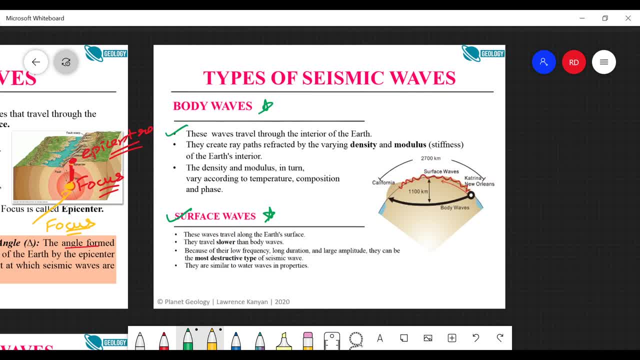 say, like on the surface. they die out very quickly, so they travel very close to the surface. so there are two types of waves. we'll study the names of these waves. okay, what are body waves? examples of body waves: you have what is called p waves and s waves. 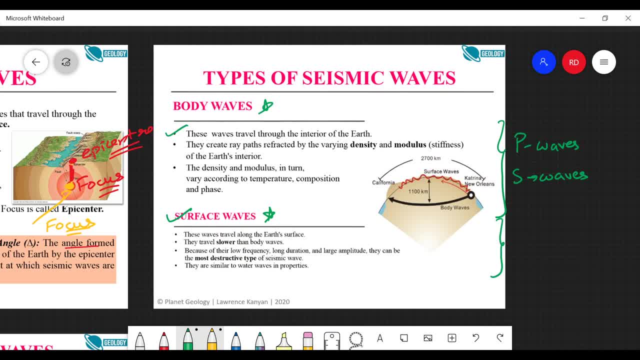 okay, so p waves and s waves for surface waves. what are types of surface waves? relay wave, love waves, l wave and r wave. okay, love waves and relay waves, rayleigh waves, okay, so this p here stands for. what does p stand for in these ones primary sir. 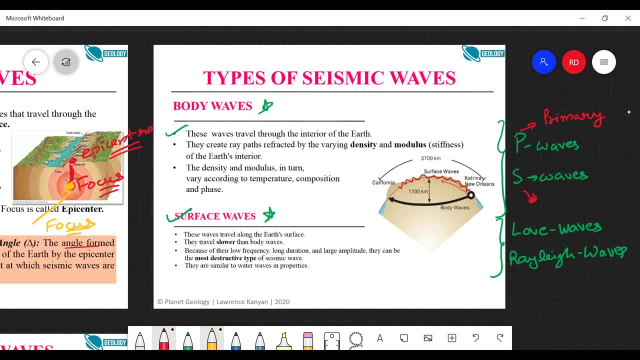 primary. because they are called primary waves? because they are the first to arrive at a recording station. they're usually the first to arrive at a recording station. that is why they are called primary waves. what are s waves? secondary waves, secondary waves, secondary waves, and sometimes you willl see that they are called primary waves. the primary waves are: 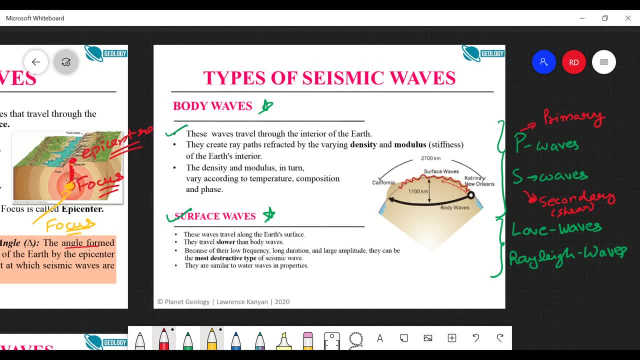 called Поэтому. you will also hear the term shear waves for s waves. okay, so, either of these. so that's why they're called s waves. okay, so body waves. you can see here they're traveling through the interior, and there are other waves which are traveling through the surface of the earth. okay, 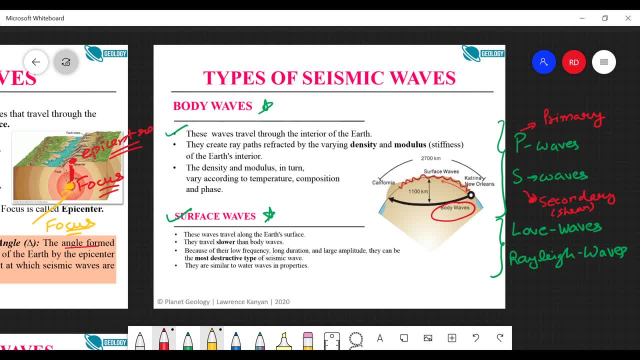 say they create ray paths that are refracted by varying density and modulus and stiffness of the earth's interior. okay, so basically, the main thing is density, modulus, stiffness. all these are changing what is called the velocity. okay, so once these waves are generated, let's say if this is the 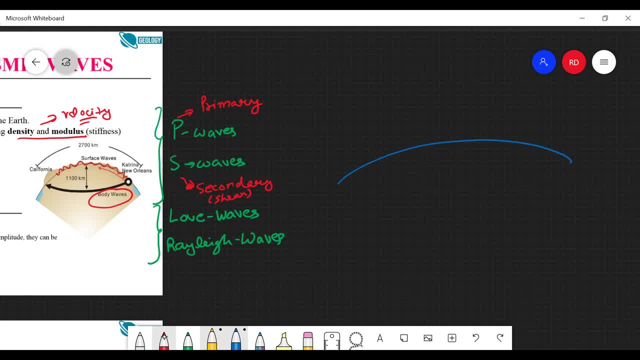 surface of the earth. they do not travel necessarily in straight lines. okay, if earthquake is generated here, it's not that the seismic waves will travel like this, okay. rather, they travel something like this: okay, they, they get refracted and some, some of these may actually be refracted. 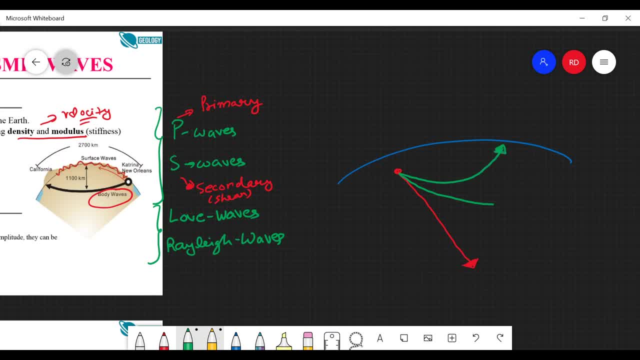 actually reach the surface okay, at some point. so they get refracted. okay, they do get refracted at some point. they may suffer critical internal reflection also. that is why they- they can reach all the way to the surface, but they are refracted and that is they don't travel in straight line. 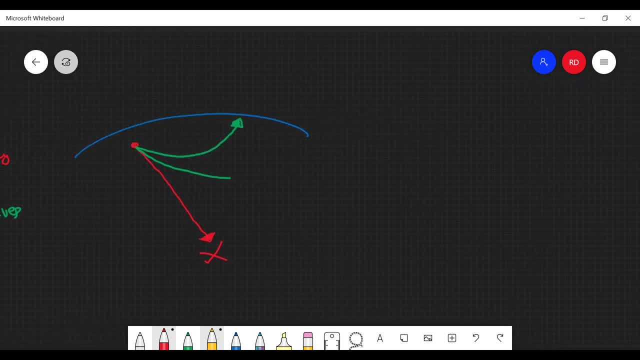 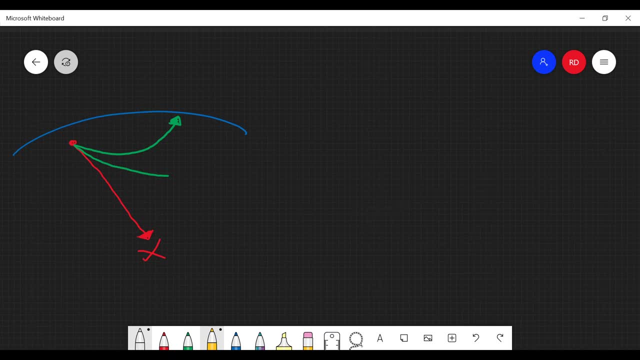 paths. okay, this is the same process you would have seen it in in when you were studying in school. how is mirage formed? okay, so on a hot day, if you're traveling on road, that on on on road, it seems that there is a pool of water, or sometimes in desert. you will see there. 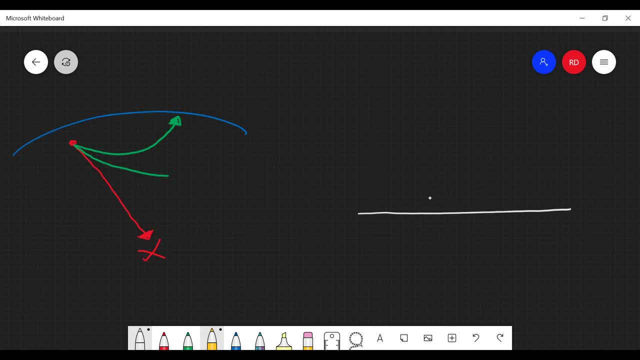 is lake. so what is really happening over there is that you have raw, you have air which is very hot close to the surface and it it becomes slightly again is relative here. it doesn't mean it's it's cold, it's just like it. in comparison to the, to the air very close to the surface, it's slightly. 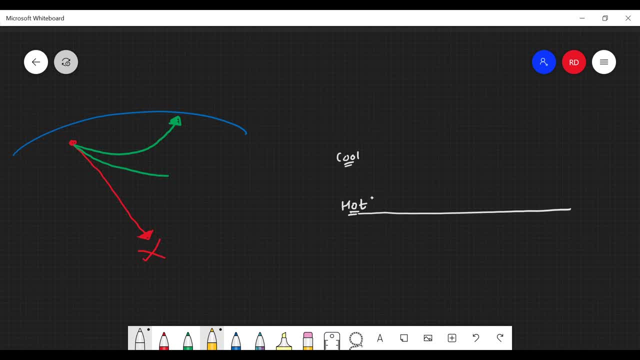 cooler, so hot air means it's it's more rare, okay, and higher velocity, so light travels at a higher velocity through hot air. Okay then then, in comparison to cooler, cold air. so what will happen is all the ways that that come here, they are deflected away from the normal and then at some point, critical internal reflection happens and it 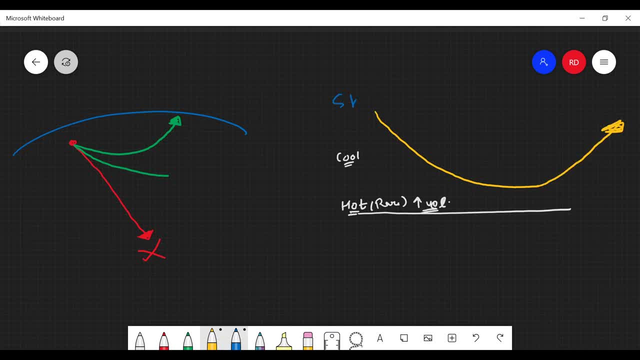 reaches your eyes and because this light is coming from the sky, you see a sort of a reflection of the sky in the ground and you see, that is it iffy, that is a pool of water on the road. okay, because you see this reflection of sky, so you have low. 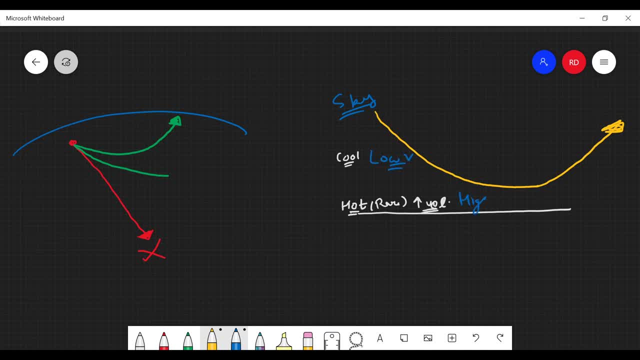 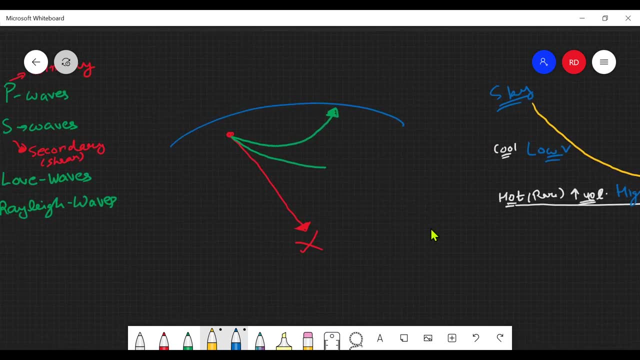 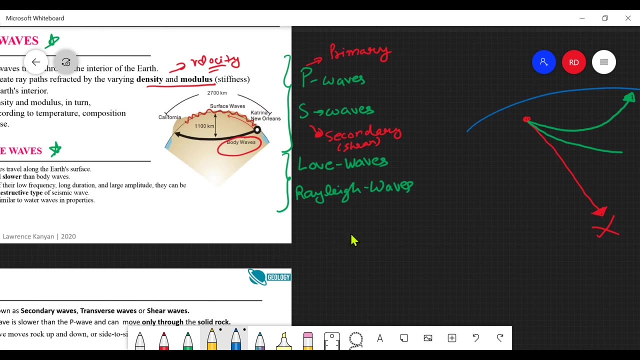 velocity. you have high velocity close to the surface. okay, it's the same process for seismic waves, because velocity of waves it will increase as you go, mostly increase as you go deeper and deeper into the earth. so these seismic waves are are sort of like refracted towards the surface. 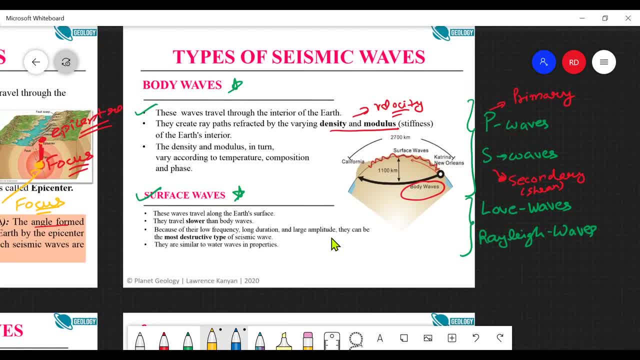 okay, so main main reason here is that it's it's due to velocity, okay, modulus and density. we'll try to understand these terms as well. so the waves: what are surface waves? they travel along the earth's surface and, again, surface waves are slower. okay, surface waves are slower than. 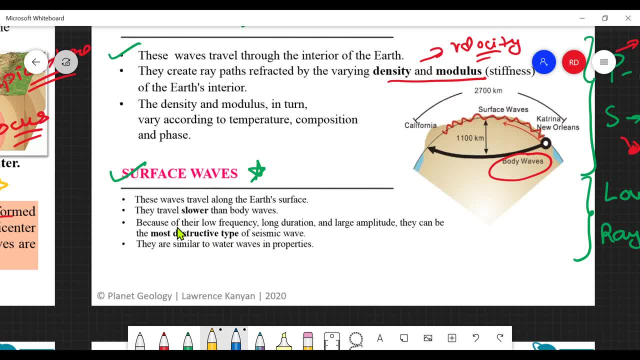 body waves. so they arrive after body waves. okay, because of their low frequency and long duration, large amplitude, they travel along the earth's surface. okay, so they travel along the earth's amplitude. they can be most destructive, destructive type of seismic waves. okay, so it's the surface. 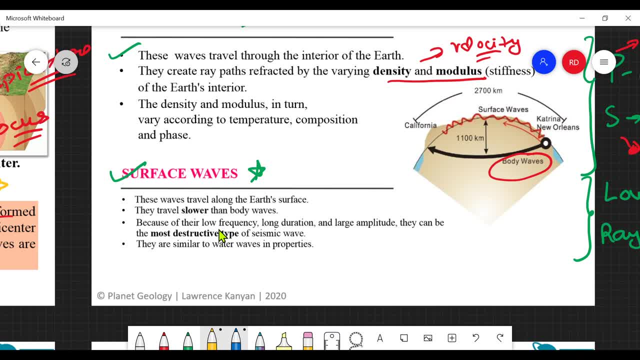 waves which are the most destructive. again, they are similar to water waves. in some properties especially, you will see the, the, the relay waves. they're pretty similar to waves that you see in water. they have large they're, they're slow, they travel at slow velocity. long duration they have. 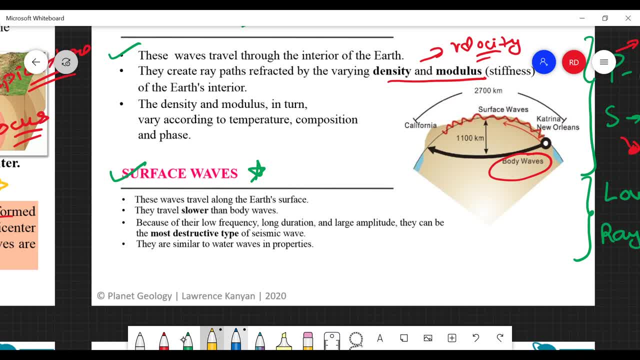 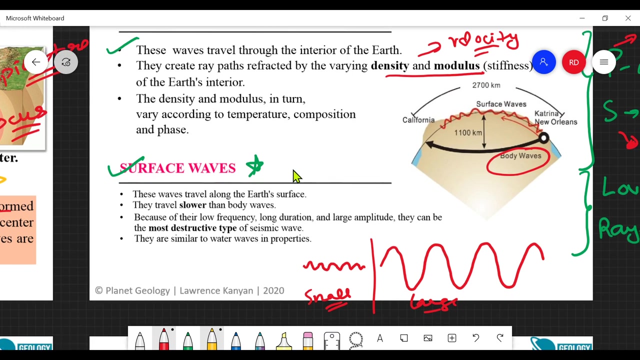 large amplitude means amplitude small if, if something is shaking, so this is what you call small amplitude and this is what you will be large amplitude. okay, so anything with small amplitude and large amplitudes, if they are with large amplitude, they will. they will, uh, uh, they will shake with a greater amount. okay, so a little bit again, very. 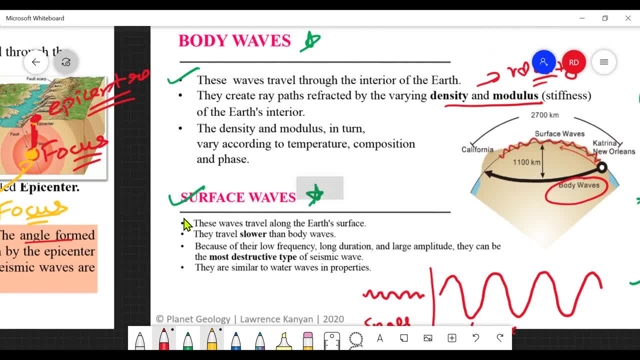 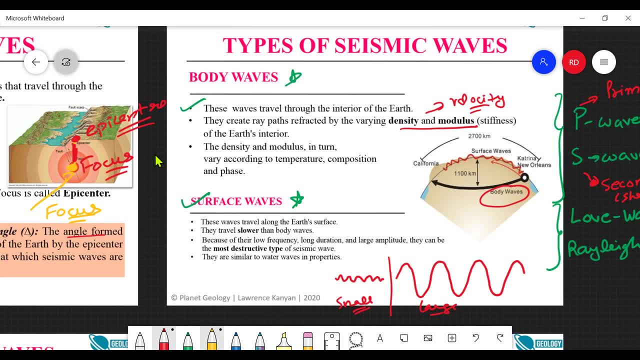 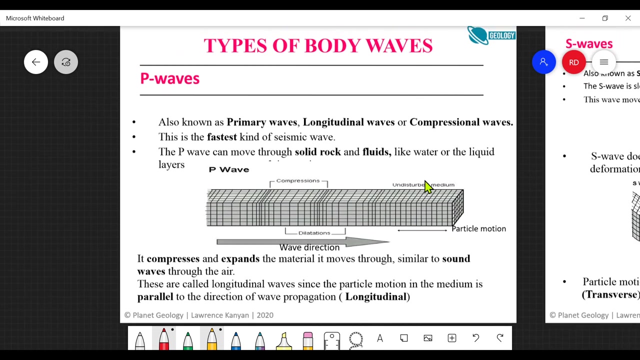 important. this question appears as it is okay, but i'm going to trivialize a little bit more. this question will especially appear during Tufts Yardwehr last year, when we hit the porous. Before we do that, are there any questions? Sir, both surface waves and body waves originate from focus. 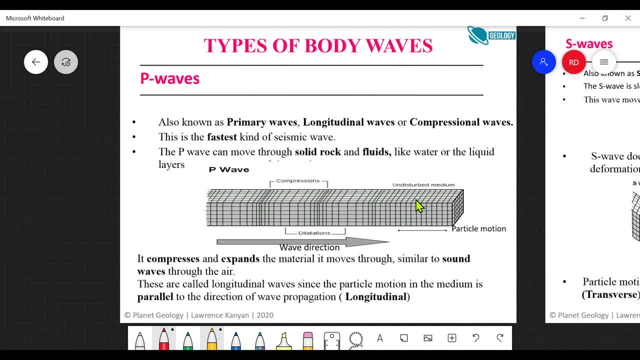 See, what happens is both the waves which are traveling on surface. if the focus is deeper, then they cannot originate from the focus, right? If focus is like 50 kilometers deep, then you will not call them surface waves. So there is a principle which is called the Huygens principle. 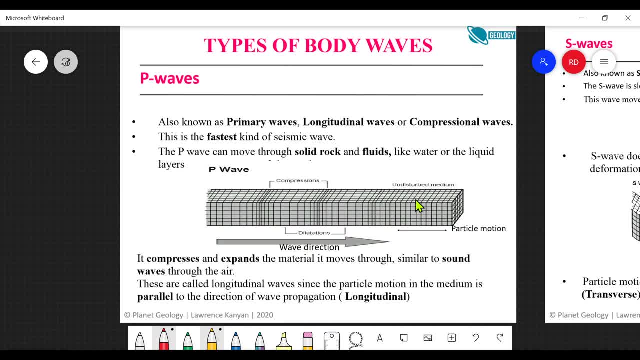 in which even a wave which is traveling through the surface, through the rocks, because it is moving the rocks slightly, it is creating a disturbance. So every point on the wave front where the wave is traveling acts as a source of its own. 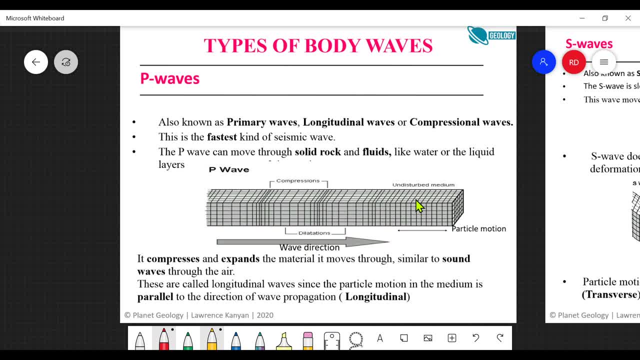 So when these waves reach the surface, they act as own source, as if miniature earthquake is occurring everywhere, And that is what results in formation of different kinds of waves. Even P wave can generate S wave. S wave can generate P wave. 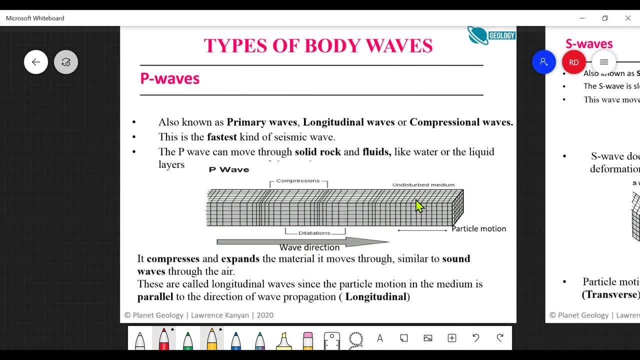 So all these things happen. So sometimes we will see secondary S waves also being generated, But these can be generated by those waves traveling, for example, P wave, S wave, So if they move through the surface, then they can generate these waves. okay. 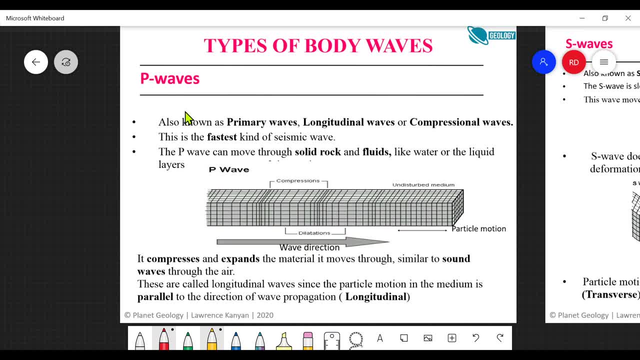 So the P waves, the first type of body waves, which are called the P waves, they are known as primary waves, also known as longitudinal waves or compressional waves. Okay, the type of longitudinal waves is very important because S waves are type of shear waves. 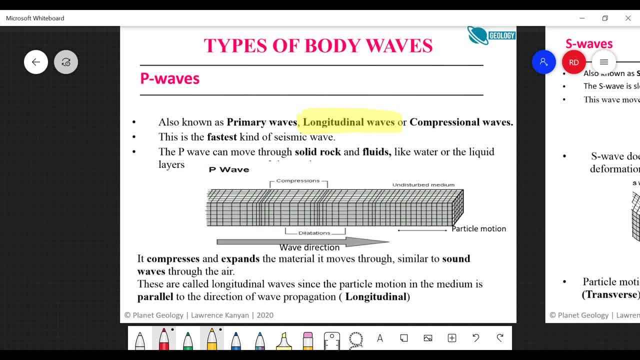 Okay, so that's why we call S waves. it is better to call them secondary waves instead of shear waves. S stands for secondary mainly because here then, if you were talking about shear and longitudinal, you could call them L waves, okay. 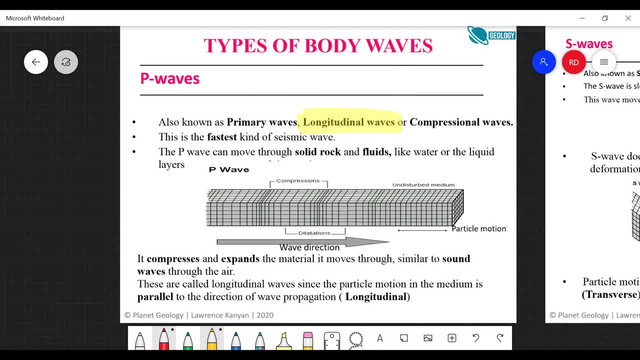 So P is for primary, S is for secondary. but it's not wrong if you say S waves are shear waves, So they are primary waves, they are longitudinal. What do you mean by longitudinal Primary waves? you call them primary because they are first to arrive. 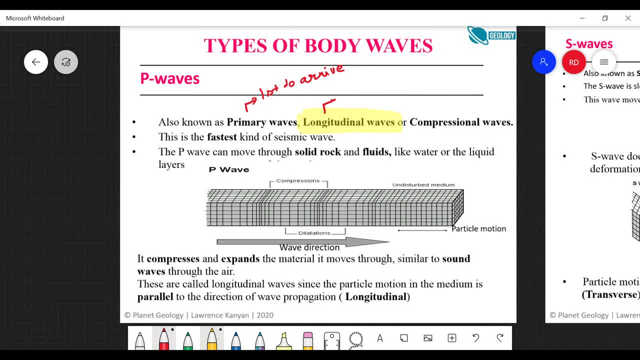 At a recording station. They are longitudinal. because why they are longitudinal? Particle motion parallel to the direction of travel Or direction in which the wave is traveling, okay, So the particle motion in which direction the particles are moving. so you see dilations and compressions here, okay, 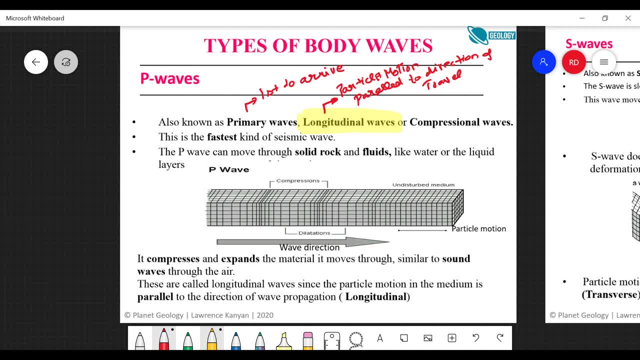 So what you actually see, these two are our dilations. okay, So these two are dilations, alright, and these two are compressions. The blue ones are compressions here. okay, So the particle motion is basically to and fro in this direction. 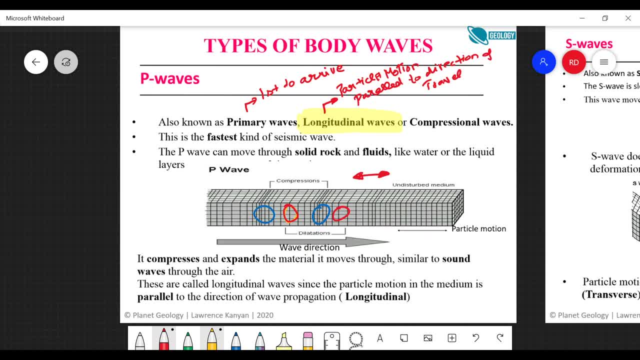 So if there is a wave, you will have the to and fro particle motion, okay. So this particle motion is in this direction, Okay, And the wave is traveling, let's say, in this direction. So the blue line is direction of travel. 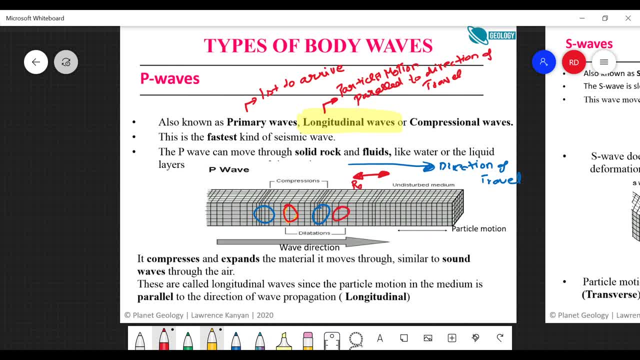 And this red line is the particle motion. Okay, So it is parallel or anti-parallel to the direction of travel. Okay, And they are called compressional waves because if, let's say, material is moving in a given direction. 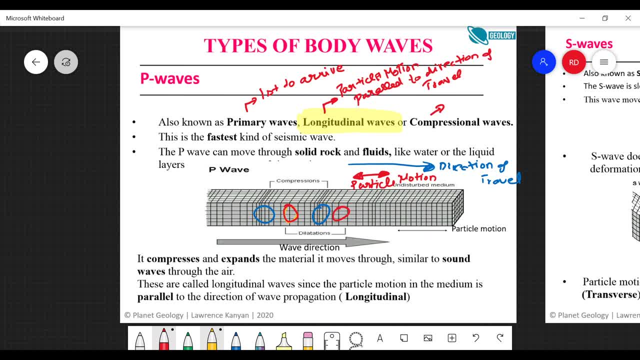 it will compress the rocks in that direction, okay. And then when it passes, then there is a, let's say, equivalent to a trough, then there will be expansion, okay. So that is why they are known as compressional waves as well. 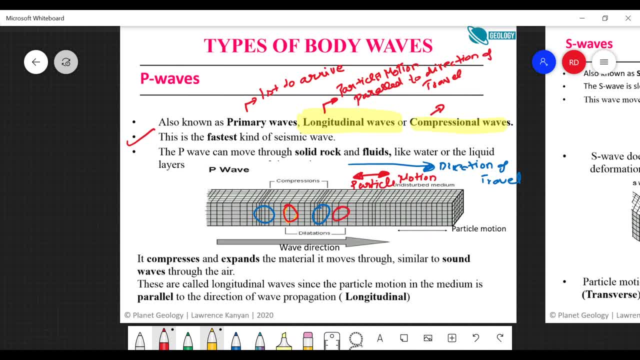 These are first to arrive, so they are the fastest. Very important. they can move through solids and fluids. They can move through solids as well as through fluids, okay, Like water or liquid. So when I am speaking, okay, when I am speaking. so now you guys are hearing over the internet. 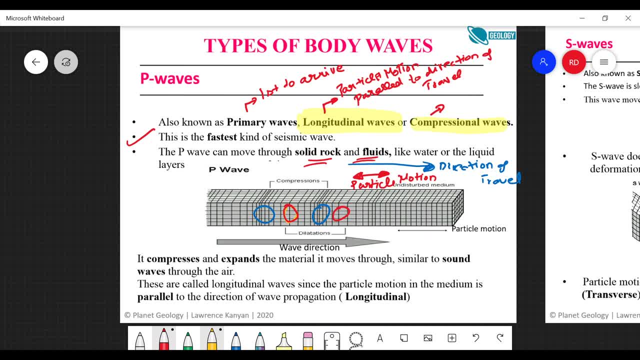 but if someone is sitting in the room with me, so what kind of waves they are listening to? Are they P-waves or S-waves? P-waves: They have to be P-waves because P-waves can travel through solids, liquids and gases. 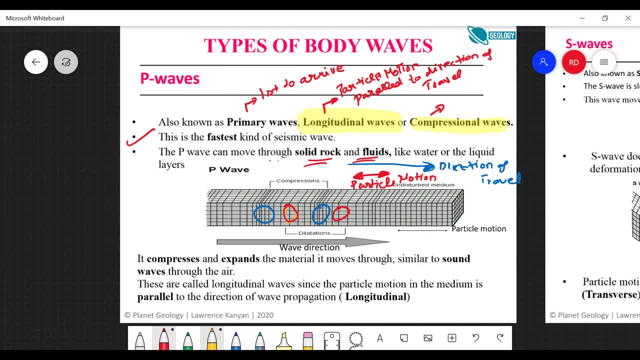 S-waves. we will study them in coming. they can only travel through solids. They cannot travel through liquids and gases. So if you are speaking, you cannot hear. So there can be no shear waves in. there can be no shear waves in fluids, okay. 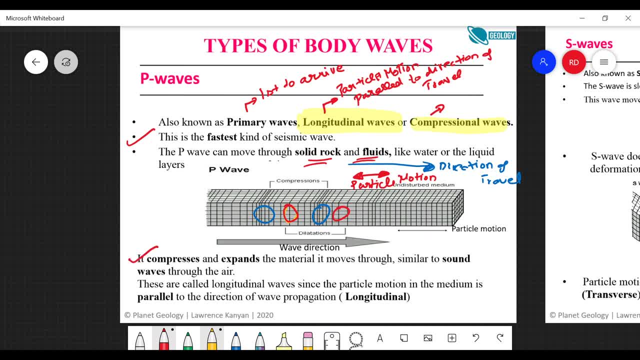 We will see why that is the case. okay, So we see this compression and expansion in these materials. These are called longitudinal waves because particle motion in the medium is parallel to direction of wave propagation. That is longitudinal. So if particle motion is perpendicular to the wave motion, okay. or the direction of propagation of the wave. 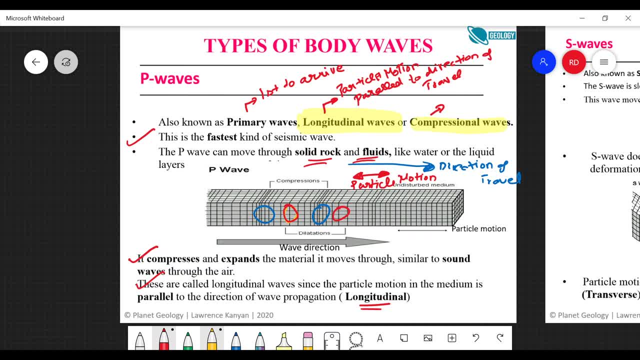 if particle motion is perpendicular, these will be called actually not just shear- waves- longitudinal and shear, it should be called transverse waves. okay, Light is light a type of transverse wave or a longitudinal wave? Sir, it is electromagnetic waves. 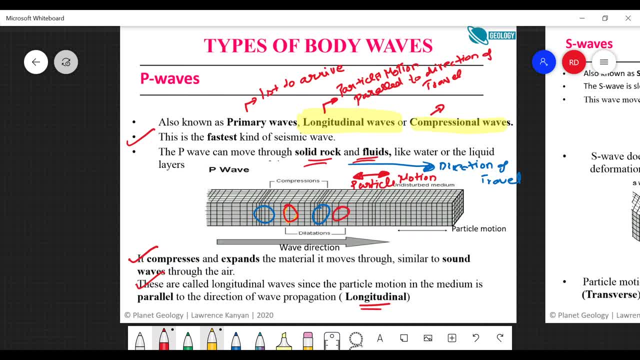 They are electromagnetic waves, but are they transverse or longitudinal? They are transverse. They are transverse Because the electric field and magnetic fields, they are vibrating in directions perpendicular to direction of propagation of the wave. okay, So this is again very important. 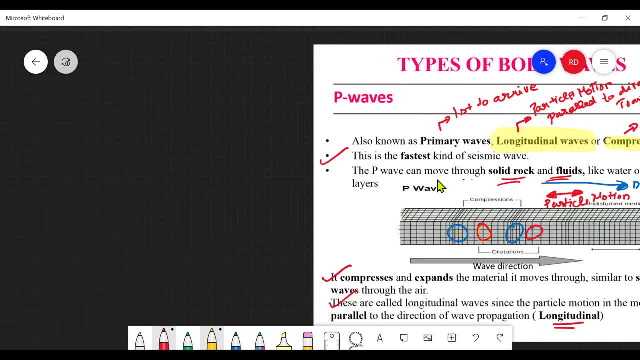 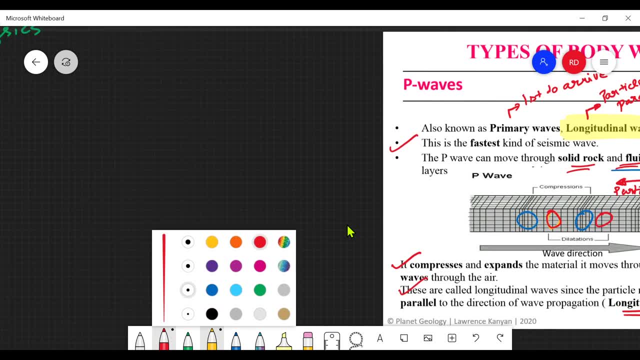 Now probably I think those things are not there in the slides again important. So I will tell you about few formulas of velocity. So I think some of you already know that part of propagation for P waves and S waves. You should know those formulas. 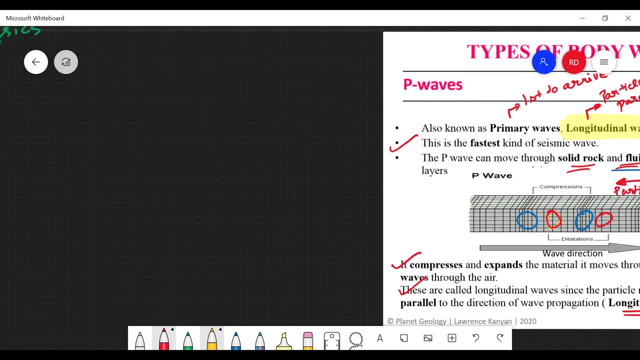 So if you are writing GSI or UPSC civil exam, they may not ask you to solve a numerical based on those formulas. but if you are writing your answer for P waves- what are P waves? you also have to mention their velocity. and how do you determine the velocity? okay, 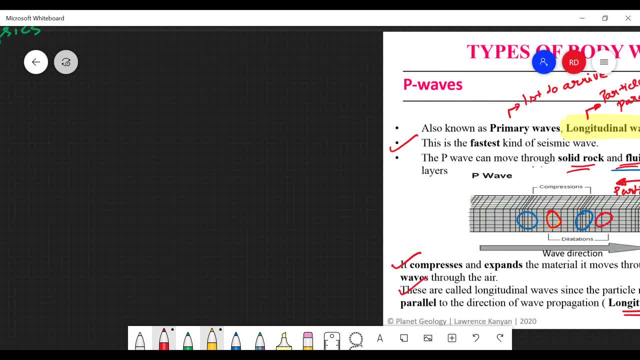 Or how does the velocity change based on the changes in properties of rocks? okay, So P wave velocity written as Vp: what is the formula for P wave velocity? Exactly, that is the formula. okay, So here, what is K? 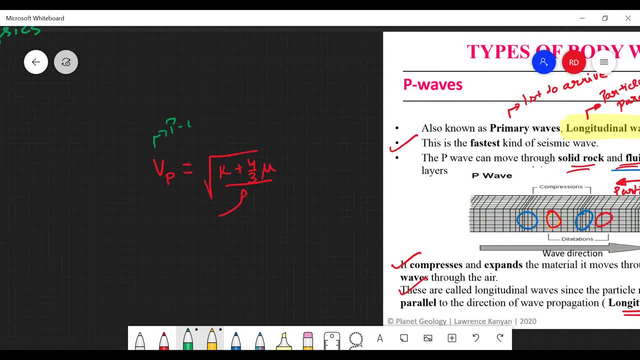 So Vp is P, wave velocity. you know that This is P wave velocity. What is K? This is the bulk modulus. I will define these, do not worry. What is mu? Pure modulus, Or sometimes we will hear the term rigidity. 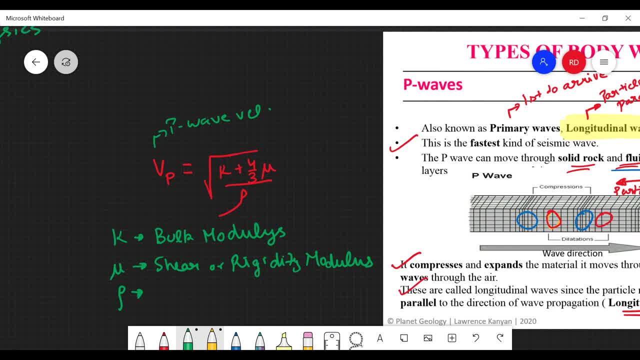 Okay, What is rho? Okay, So rho is density and rho so you these. these are the terms here. what is bulk modulus? now someone may ask you the question: what is bulk modulus? how do you define any kind of modulus? okay, so, very simply. 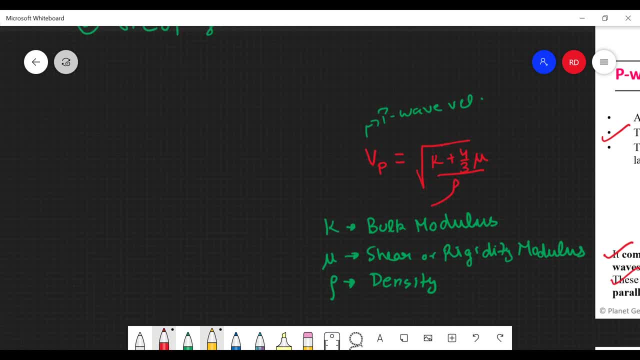 yes, sir, it is a ratio of volumetric stress to volumetric strength. yes, exactly so. bulk modulus k here is equal to volumetric stress over volumetric strain. okay, so all these kind of moduli, that you will see, they, they generally arrive over there because you know that stress. 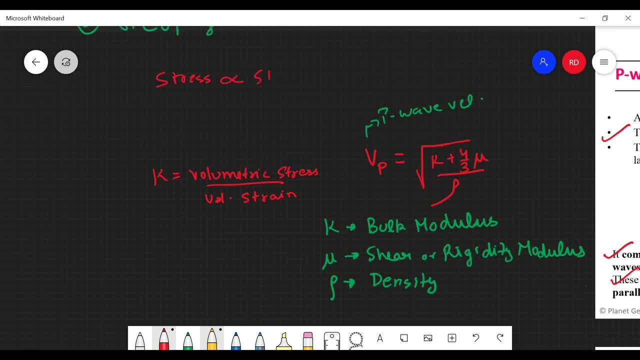 in a rock is directly proportional to the strain. okay, so strain, so stress, is directly proportional to the strain. okay, so the greater the strain means strain is basically deformation. okay, what is strain? strain is basically ratio of change in dimensions. if you are talking about why. why do we use the term volumetric here? because we are talking about 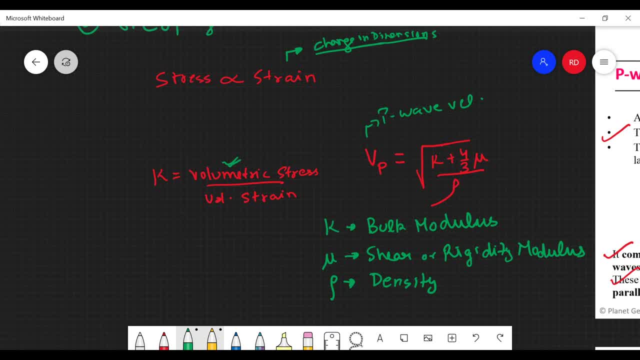 the dimension we are talking about is volume. you may talk about someone may talk about length, okay, so change in dimensions divided by some original dimensions, okay. so if you talk about linear strain, okay, change in length divided by original length, that will. that will be what you call linear strain. volumetric strain will be change in the volume. 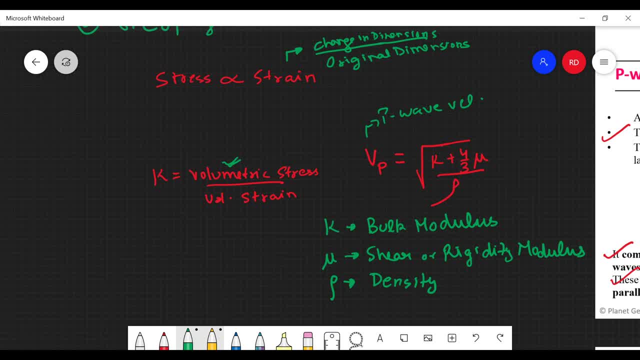 divided by original volume. okay, stress again, i will not go into details. it is actually what we call a tensor. okay, so a tensor, as you know, is very, very famous beyond any, but overall you can think of it as equivalent to, to, to. it's not pressure, it's not. you can think of. 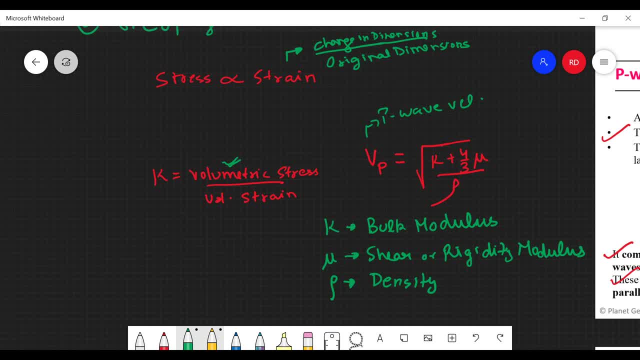 it as force per unit area and then for for a given plane. okay, if you have a plane, what is a force per unit area? it will depend on orientation and all there are other things, but overall it's it's force per unit area. okay, so that that's what, what you will have, what we'll call stress, so volumetric. 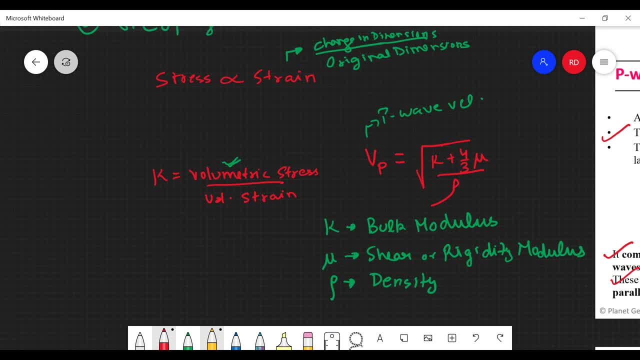 stress, or stress is directly proportional to strain into bulk modulus. okay, what is rigidity modulus? so what is bulk modulus? let's say you have a sphere you compress, try to compress it. okay, so it will get smaller. okay, so there will be some change in volume if it resists. 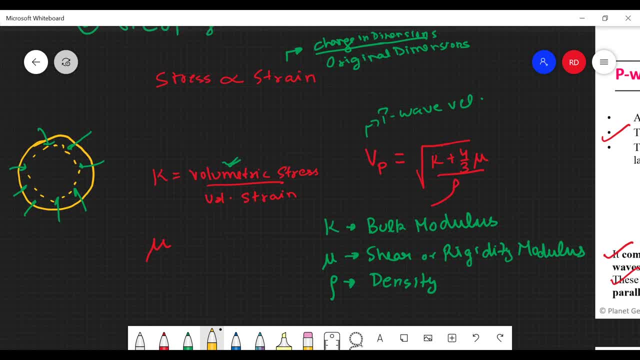 that change in volume. it will have high bulk modulus. okay, so for for you will require a lot of stress to change the volume by a little bit. it means it has a very high bulk modulus. so if k is high you can see stress equals to k into strain. so strain will be change in volume. 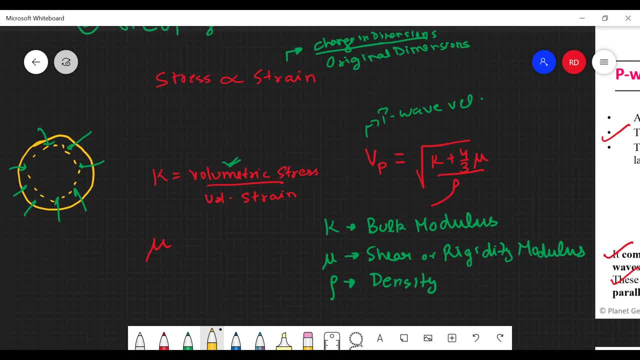 okay, divided by original volume. so to produce very little change in volume you will require a lot of stress. that is what is the bulk modulus. that is what bulk modulus is. mu mu is the rigidity modulus, because it is. if rigidity modulus is high, it means that that particular body will resist. 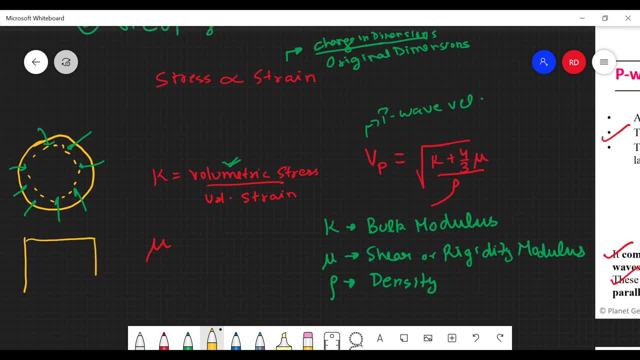 change in shape. okay so if, if you have, let's say, this rectangle here and you want to change its shape, okay so you apply a force like this. okay so, if something has high rigidity modulus, it will resist that change. okay. so again, in which, in this particular case, if you have a high rigidity modulus, 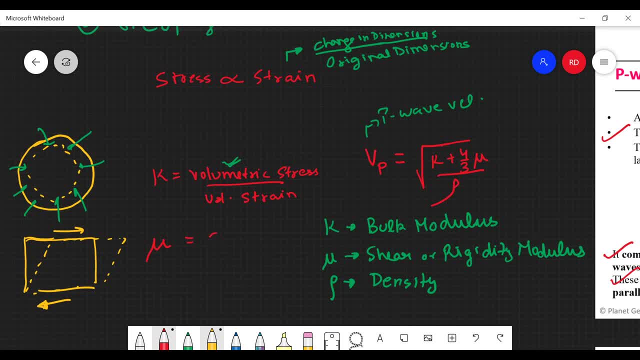 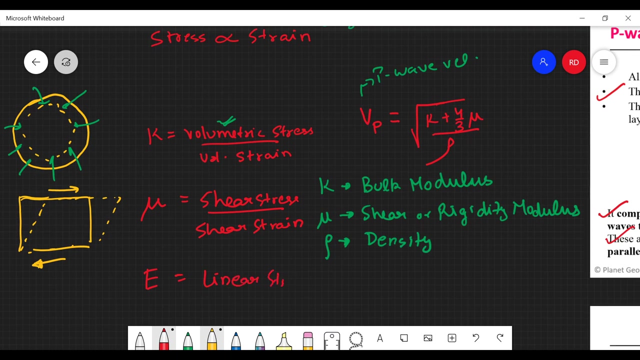 it will be what what we call shear stress over shear strain. all these moduli are basically ratios of some kind of stress divided by some kind of strain. you can have young's modulus also. okay, that will be linear stress over linear strain. so this is young's modulus. 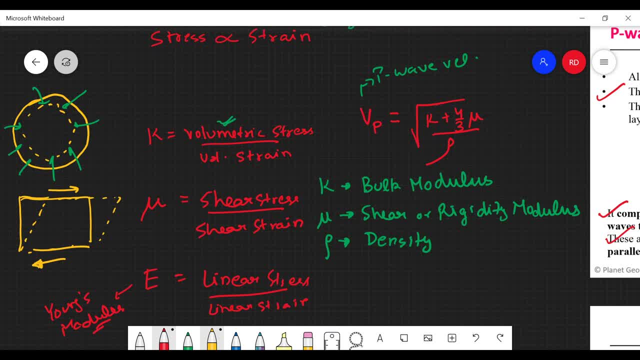 okay, so this, this is what what we have in here now. shear stress is again important to understand here. so, for example, if you have, uh, let's say, a balloon with you that's a gas or a balloon filled with water or air, whatever it is, if you try to compress it, do you feel any? 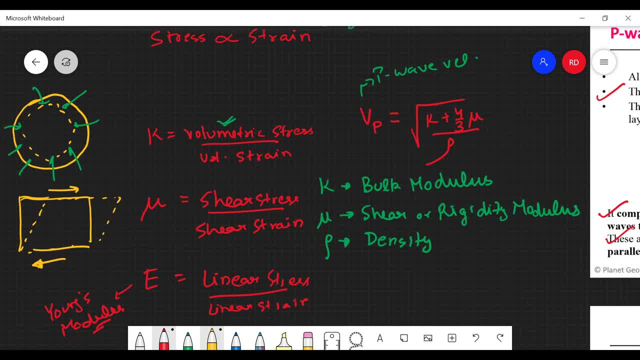 resistance which you have, because, as we just talked about, uh, if you do, don't suppose you do clearly feel any resistance. you do feel resistance. right? if you cannot, you cannot compress it beyond the value. so everything has bulk modulus on some of the things. okay. now what about shear modulus? okay, 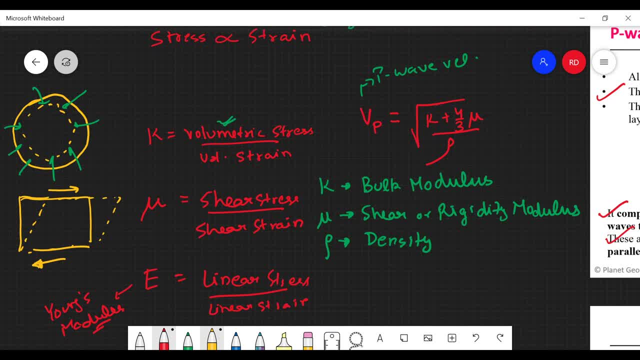 let's say, if you place your hand on top of a table and you try to move the table, what will happen? can you move the table buy by sliding on on top of the table? your hand will try to resist that change. okay, it will apply force in opposite direction, so it has a fixed shape. 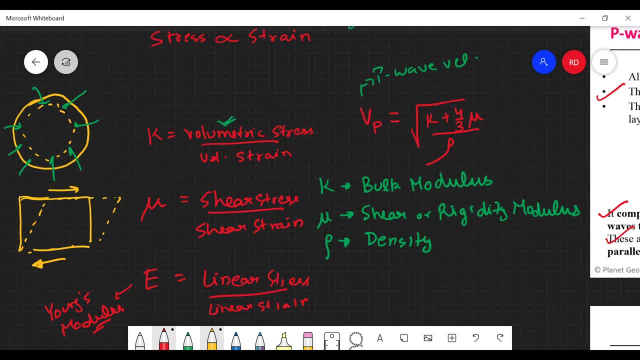 okay, if something has a shear modulus, it means it has a fixed shape. it has a shape because it resists deformation. gravity is acting on all the bodies, okay, so there is some force on all the bodies. so there is some deforming force in there, but some of some, some stuff, for example, your table. 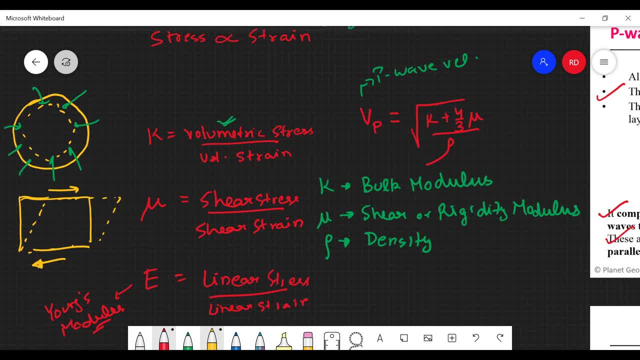 chair. they have fixed shape but there are some materials which do not resist any change in shape. if you move your hand on top of water, there will be no. water will not resist. there may be drag. water is moving out to the sides. but you cannot in a beaker. you cannot put your hand and try to. 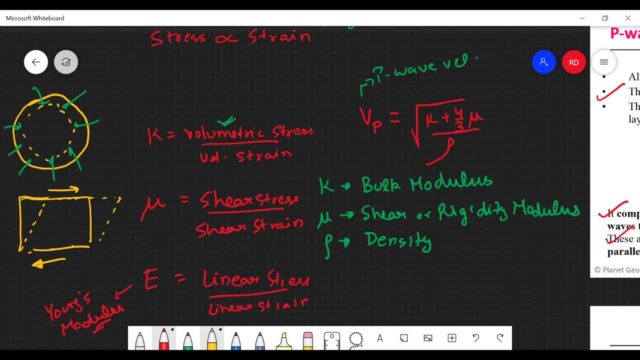 move water and that will not move the beaker, okay, water will just flow according to the, according to the movement. okay, and that is why water at as well as gases, they do not have any fixed shape. they acquire the shape of the container in which they are put, because they cannot accommodate any. 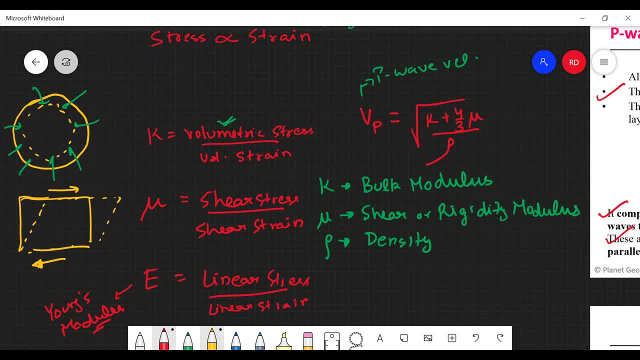 shear stress. you cannot have any shear stress in water because mu is equal to zero for fluids. okay, zero for fluids. what do you mean by fluids? fluids means liquids plus and lower liquids and gases. okay, so again very important to to to understand this part. now, how do we? 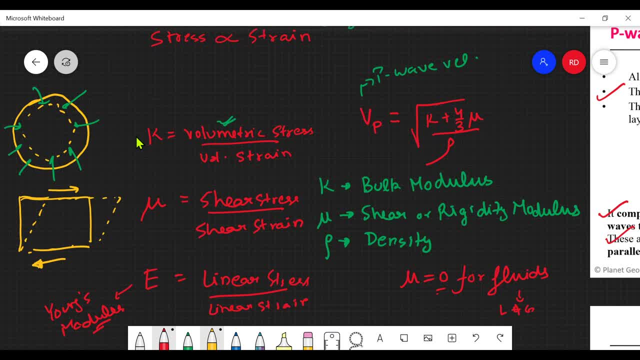 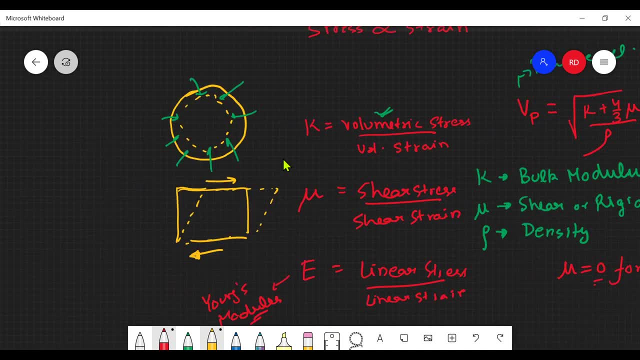 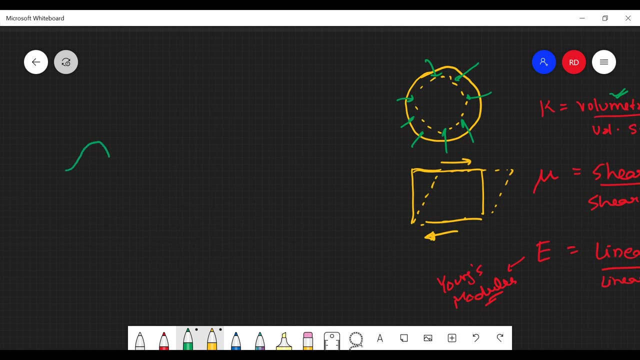 actually travel. okay, that is also you. you need to understand. okay, so why do you get a wave in the very first place? okay, so wave waves are generated. let's say, you have a rope in which you're trying to generate a wave. okay, if this rope is, let's say, stretched, it's well stretched between these two. 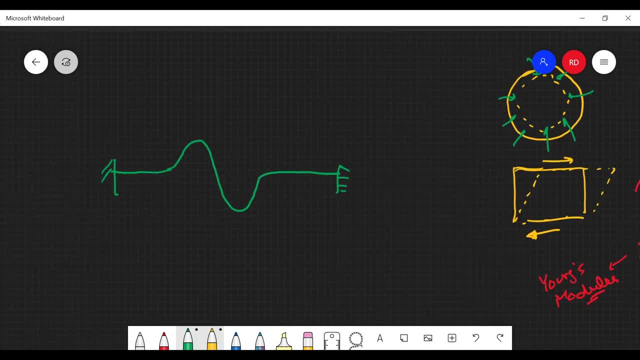 points? okay, it wants to stay straight. okay, but when you deform a particular part of it, okay, let's say when, when this particle moves up? okay, now this, this, uh, this rope- it gets stretched. okay, what happens when? when a rope gets stretched, it will pull back, okay. so when this particle moves up, there is a force in the opposite. 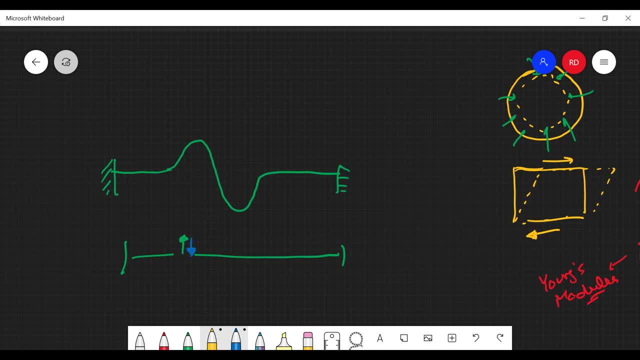 direction which is pulling it down. okay, very important to understand. so this force which is acting in the direction opposite to the particle motion, and usually it is proportional to to to that displacement, so you need that force to generate waves, that that resisting force has to be there. that is why this part will come down, okay, only then, and then it can overshoot it. 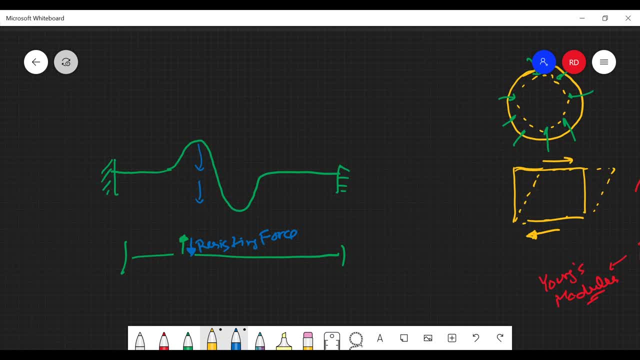 can go all the way, also in some cases, so that resisting force has to be there. so this is displacement, the green arrow, this is displacement, and then it can overshoot, it can go all the way. so this is displacement of the particle, again very important, for example in in displacement of 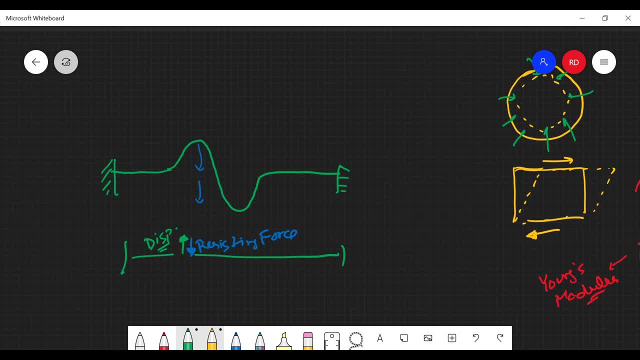 particle and direction of travel of wave are two different things. okay, so particles may be displaced in whatever direction possible. direction of travel is entirely different. okay, so where will this wave be next? okay, this, this wave could be next at this point. okay, particles are not moving in that. 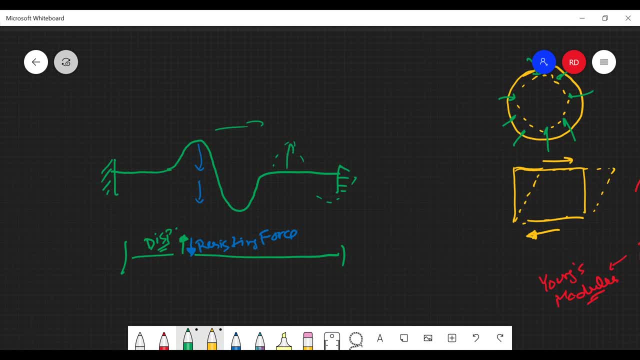 direction. only energy is being transferred in that direction. particles are still moving to and fro in direction perpendicular to direction of travel. okay, so this is displacement of the particle and direction of travel. so there has to be a resisting force. if there is no resisting force, there will be. 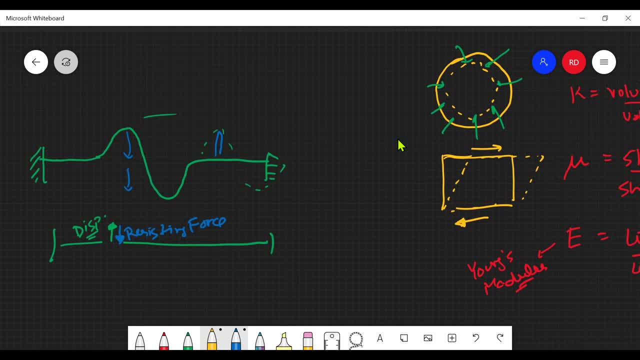 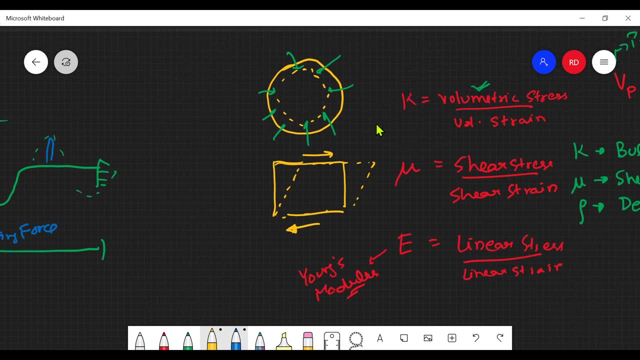 no wave. you understand this part, and what we just learned is that canned liquids, so this moduli that we are talking about, bulk moduli, rigidity moduli- they are basically resisting. the bulk moduli is resisting change in volume, the shear moduli is resisting change in shape. so for, if so, what happens? 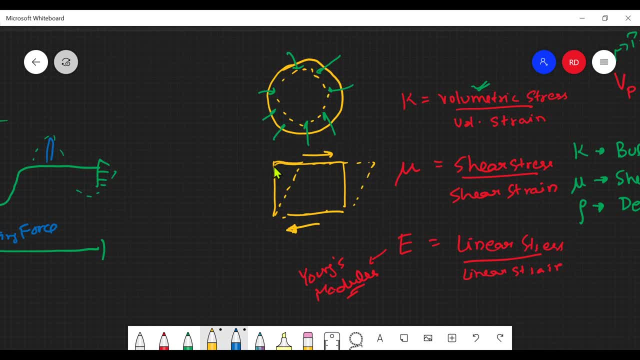 for for liquids and gases, do they have any shear moduli? it's zero, it's it's zero, right? so what does that zero shear moduli means? is means that if the shear modulus is zero, it means that there is no resisting force. okay, there is no resisting force. and if there? 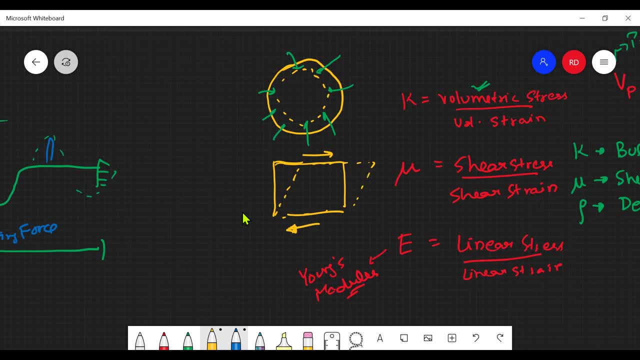 is no resisting force, what will happen in that case? those particles, if you move? okay, even if there is pendulum, right, you want to swing a pendulum, because of gravity, it wants to come back to its equilibrium position. okay, if there is no that force which which is trying to pull it back? 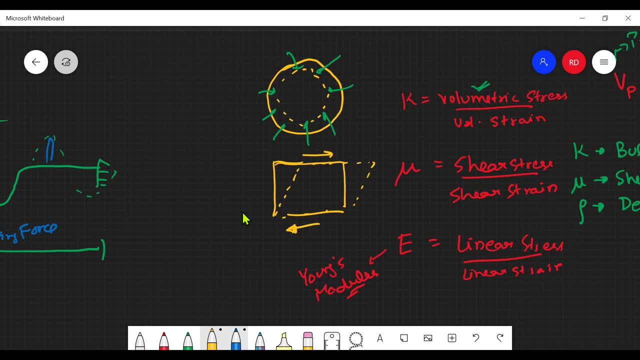 then there will be no wave. and the reason that there are no s waves in case of, in case of liquids and gases, is because they do not resist this change in shape. they do resist change in volume. so that is where they do have p waves. they do transmit p waves, but they do not transmit these kinds of waves. 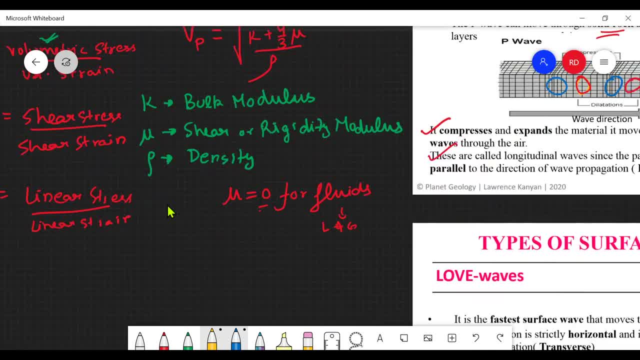 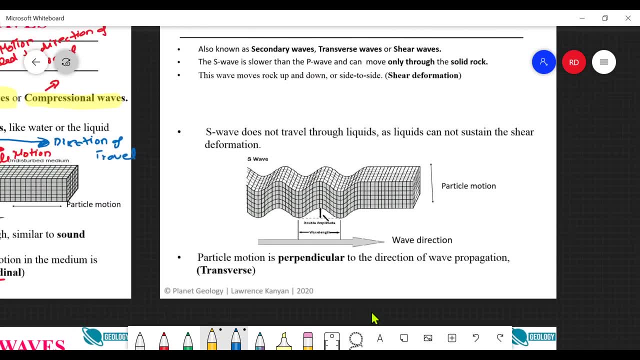 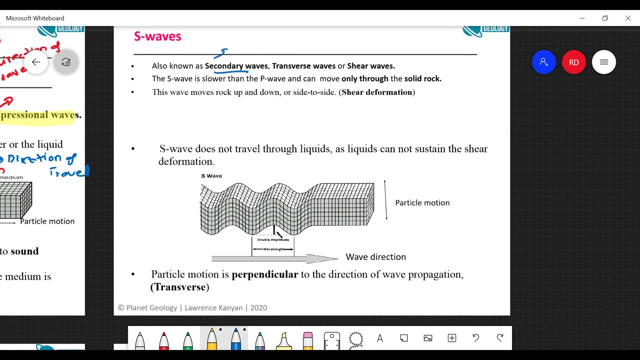 okay, s waves are not transmitted, so this, this again, are important. this is what we see in case of s waves, also known as secondary waves. okay, because they they arrive after p waves. p waves were longitudinal. these are transverse means. particle motion is perpendicular to propagation direction of wave. 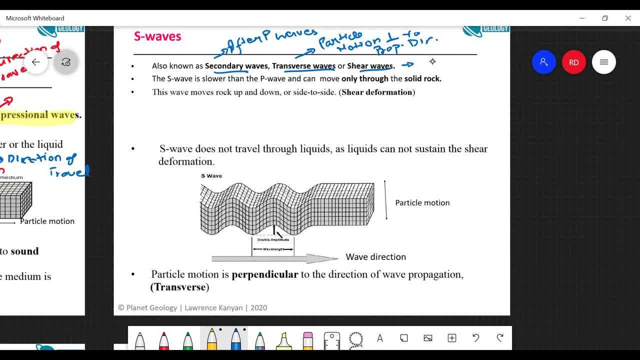 okay, shear waves, because they rely on shear modulus, or the shearing properties of the rocks. s waves are slower than p waves and can move only through the solid rock. these waves move up and down or side to side. okay, so they move up and down and necessarily it's, it's not that you will only have s waves moving. 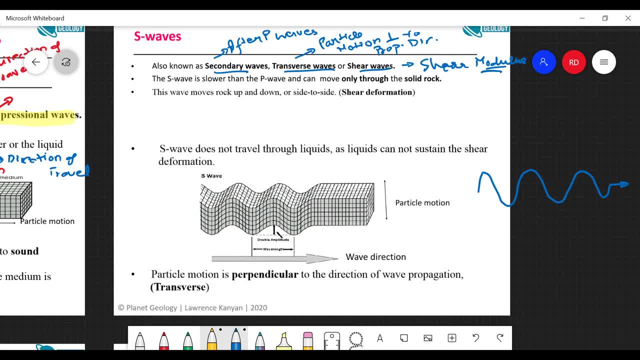 like this: okay, they can actually be moving in all directions perpendicular to the direction of propagation, for example. even this direction is perpendicular. okay, there may be other direction, even this direction could be perpendicular. okay, so some some something in in between these. okay, so all all the directions which are perpendicular, okay, so what you can think of it is as a sort of 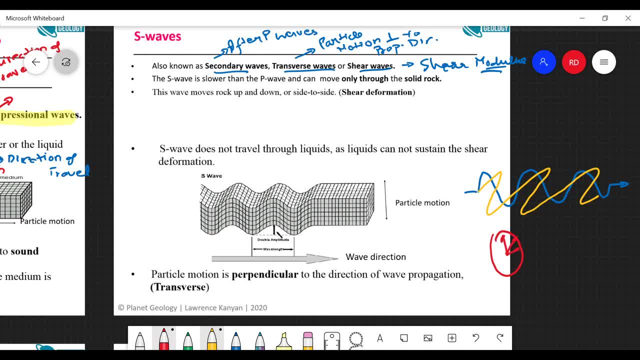 a plane. these are vibrating in all these directions. okay, they may be vibrating on all those directions which are perpendicular to this direction of travel. okay, so all the directions are perpendicular to the direction of travel. so shear s wave could be vibrating in all those directions, because here we don't have a rope. okay, just rope. we. 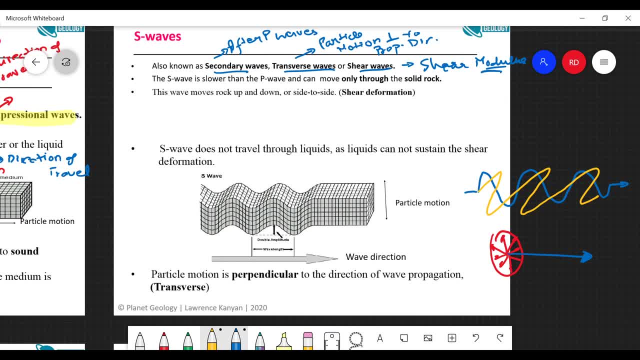 have actually ground material and it could be vibrating in all those directions. what is the formula for velocity of s waves? we have already seen for v? p waves. i will write it again. for p waves, it was k plus 4 by 3 mu over rho. for v? s, it is square root of. 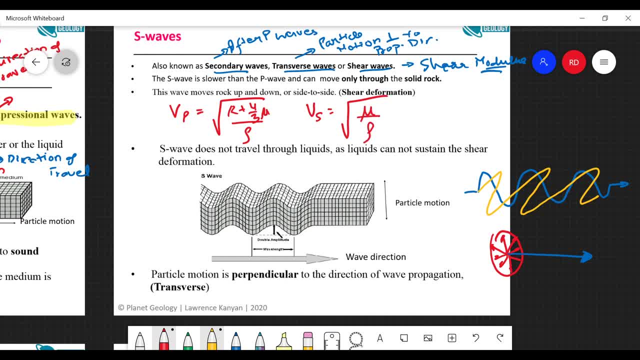 mu by rho, just mu by rho. okay, it's just square root of mu by rho. so if mu equals to zero, v s equals to zero. v p is not equal to zero, because there is still this k over there. okay for v? p. if mu becomes zero, v s becomes equal to zero. the particle motion is perpendicular to direction. 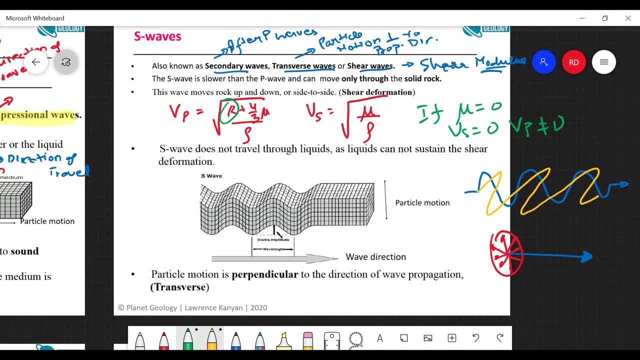 of wave propagation, again very important. now you have already seen both these formulas. okay, you. where do you see density? with density, it appears in the denominator. so if density increases, if density increases, what will happen to p and s wave velocities? will they increase or decrease? they will decrease, okay. so what happens to density as we go to go deeper and deeper into the earth? 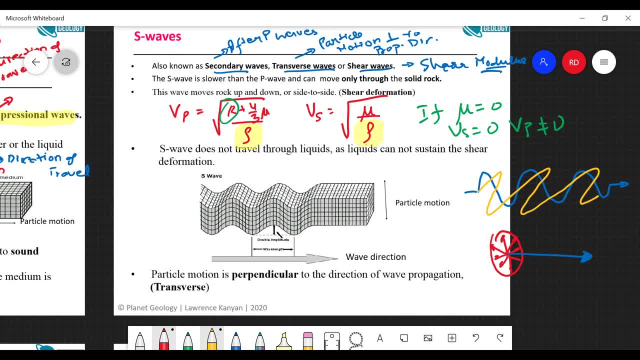 sir. density will increase. velocity will increase. why will velocity increase with density? density is it's appearing in the denominator right and its value is hugely greater than one right. so the thing is, density increases as you go deeper into the earth and deeper into the earth. so v? p and v? s should what they should decrease. 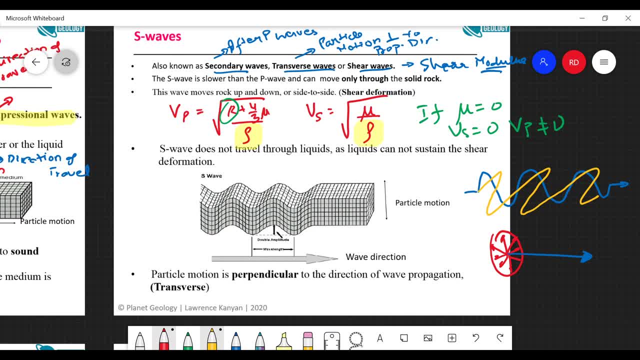 decrease. what again they increase? yes, they increase. yeah, you are correct. why, then, why do they increase? what is the reason for that? so, due to increase in density, the value of mu increase more. yes, yes. so because you have not just density in the formula, you also have this numerator. 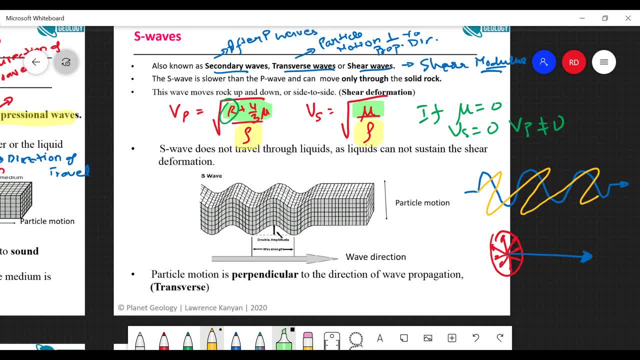 terms. okay, if the density, if, if those were constant, then yes, with density the, the p wave velocity will decrease. but what happens is as you go deeper and deeper, with change in density, you also see changes in k and mu. okay, so density increases, but k and mu increase at a faster rate, especially. 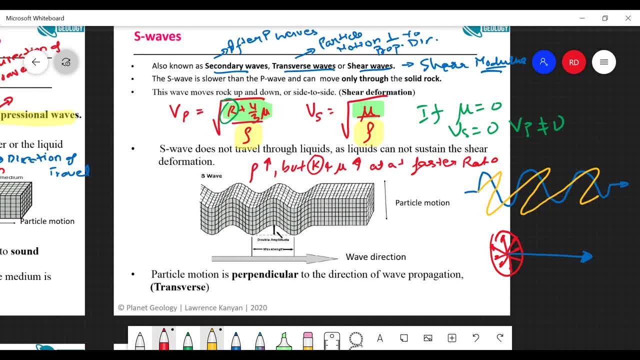 k, right especially k. mu will also decrease in some parts significantly. k can also decrease, but mu will significantly decrease. in some parts mu will also become zero. so mu does not always like increase. there are exceptions to these, but overall, the reason for increase in velocities as you go deeper and deeper into the earth- especially like up to mantle, it's the main reason- is that increase in bulk modulus- okay so- and and also, to an extent, increase in shear modulus. 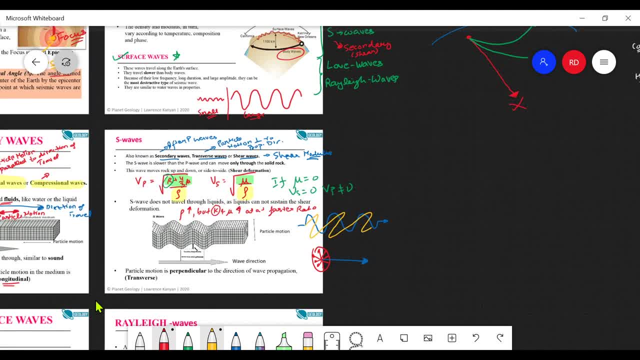 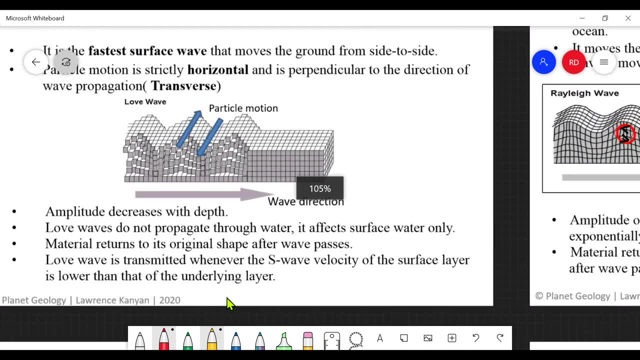 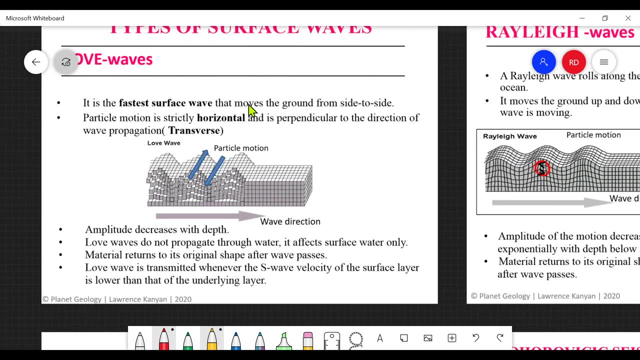 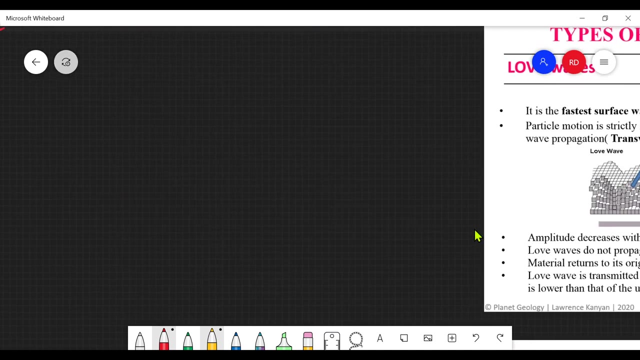 then flatter. ok, alright, so moving to the next part. then there are other types. they are Luv waves and then there are Rayleigh waves. ok, so LUV waves there the fastest surface waves. so Rayleigh waves are faster than Rayleigh waves that moves the ground from side to side. ok, so this is the difference here. 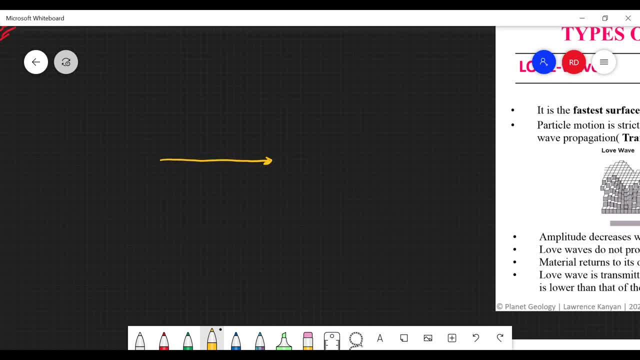 okay, when we're talking about S waves. ok, if this is the yellow line is the direction of propagation, s waves can vibrate in any direction perpendicular to it. okay, so all these directions of vibration are possible. this one, all these directions are possible. okay, now s waves. oh, sorry, what what we call love waves? you will also hear. 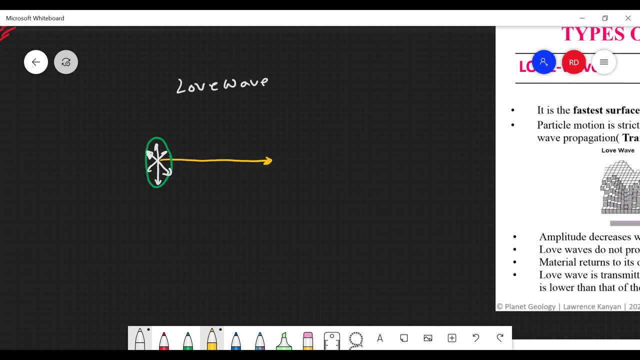 this term love waves. they are horizontally polarized. they're horizontally polarized s waves and they travel only on surface. okay, okay. so now, of all these possibilities, they are not allowed to vibrate in all directions. so this could be s wave. okay for love waves. they are allowed to travel only in one of these directions. 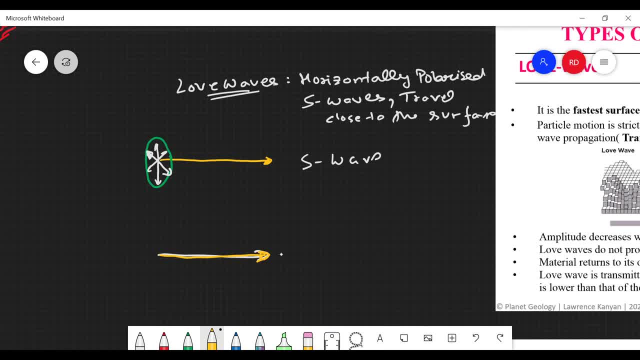 okay. so if this is my love wave, okay, it can vibrate only in this direction. okay, it cannot vibrate in other directions. so its motion will vibrate only in this direction, so it can vibrate only in this direction. will be more like this. so how do you imagine it? imagine it like a snake moving, snake moving on. 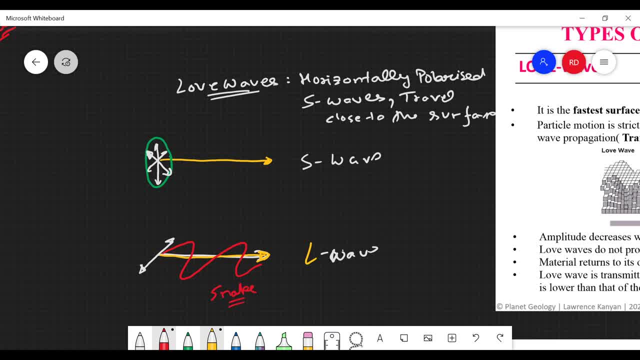 ground, okay, as if, like a snake, is moving on ground. that is what you mean by horizontally polarized- okay, just like you have polarized light, non-polarized light or non-polarized waves, they are vibrating in all the directions. in all these directions, okay, if they are vibrating in. 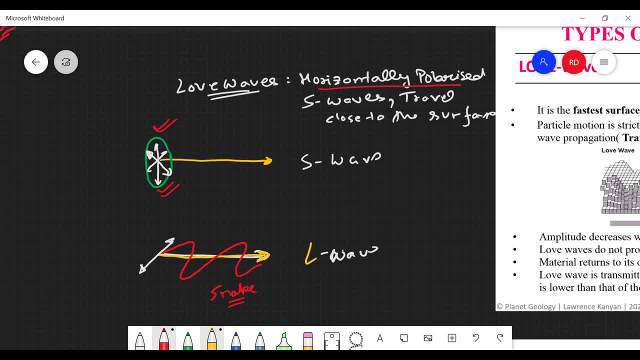 one particular direction that is called polarized. okay, that particular direction is called polarized. established direction is horizontal. in case of love waves also exist in this case are also aáticas of love waves. case of love waves. okay, so they move like, like a snake on the surface. 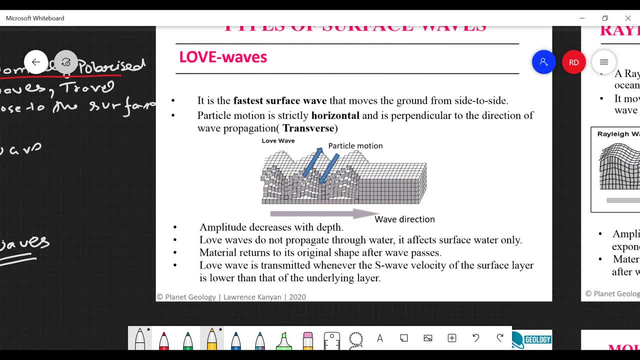 okay, so the particle motion. again, these are a type of transverse waves, only because particle motion is still perpendicular to the, to the direction of propagation. okay, so you can see this: this particle motion is still perpendicular and this is the wave direction. amplitude: amplitude decreases with depth, so 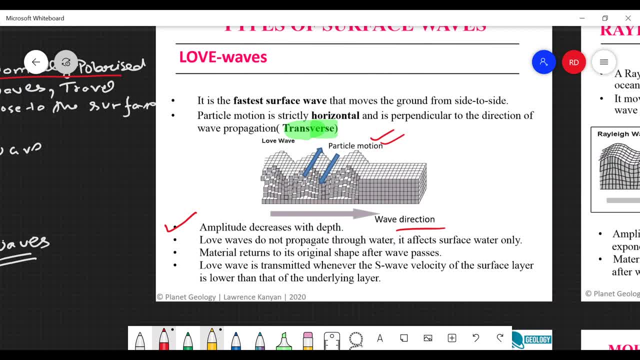 So, strictly speaking, they are not just on the surface, but they are pretty close to the surface. Love waves do not propagate through water. It affects surface water only. They will not propagate through the material, Material, surface, ground. it should be like a ground surface. 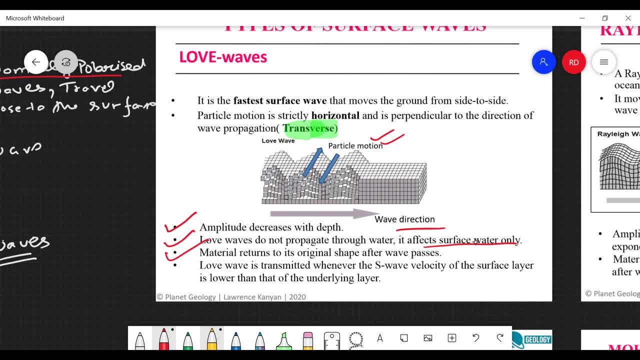 In here. material returns to its original shape after wave passes, So it affects- I shouldn't say like even it will affect- surface water, but they will not propagate through water. It will shake water if let's say there is water underground, but they will not propagate through it. 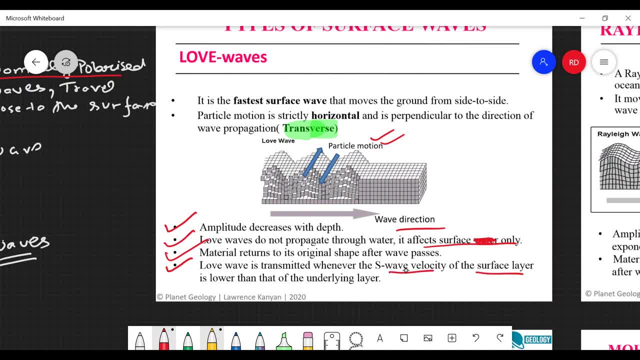 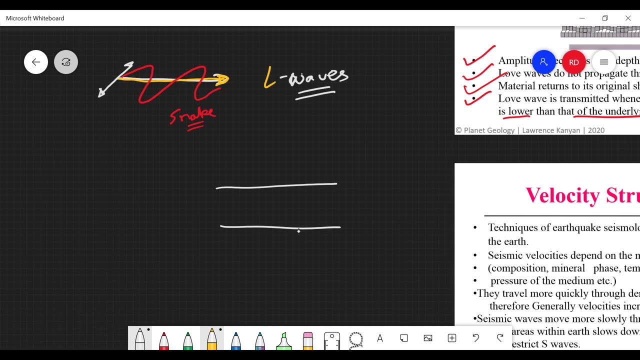 Love wave is transmitted whether S wave velocity of the surface layer is lower than that of underlying layer. So their surface waves does not mean they will only be on the ground surface, They will be on any surface. The condition is, let's say, if there are two layers in here, for surface it is basically air and rock. 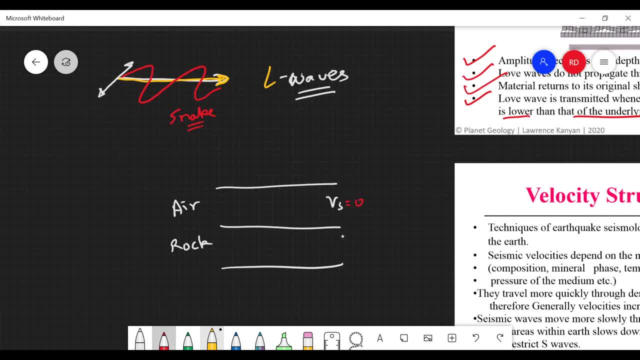 Okay, So here Vs equals to zero. Okay, So here Vs equals to, let's say, some value. Okay Is not equal to zero. And there could be another layer as well. Okay, Let's say, this layer has we love Vs. 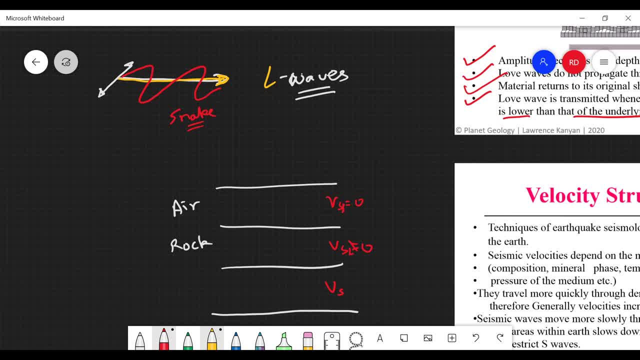 Let me call it 1, 2,. 3 is greater than Vs2.. Okay, So these love waves will be produced here as well as they will be produced here. Okay, So, whenever overlying layer has lower velocity than underlying layer, you will get love waves. 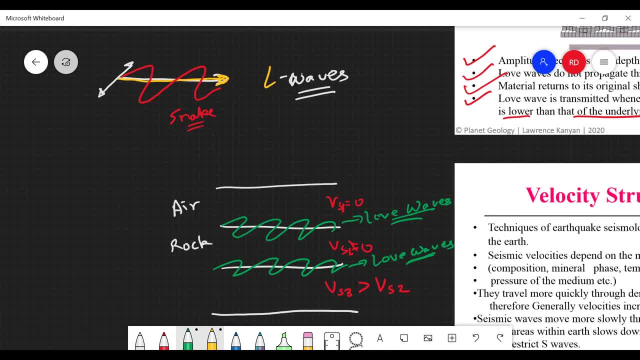 Those who are enrolled in the GATE course. we will come to this part in case of when we study Now. in the next lecture we will study sonic logging, And sonic log is a type of log which relies on acoustic waves And in there also you will generate. 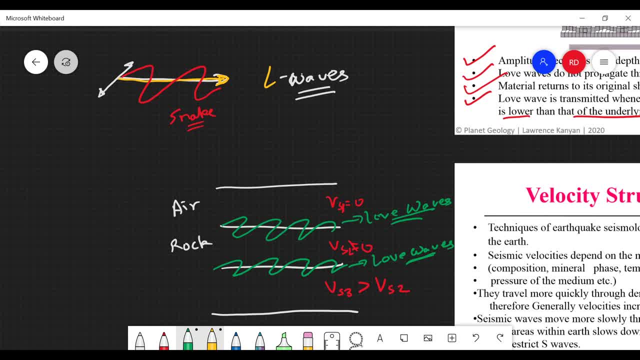 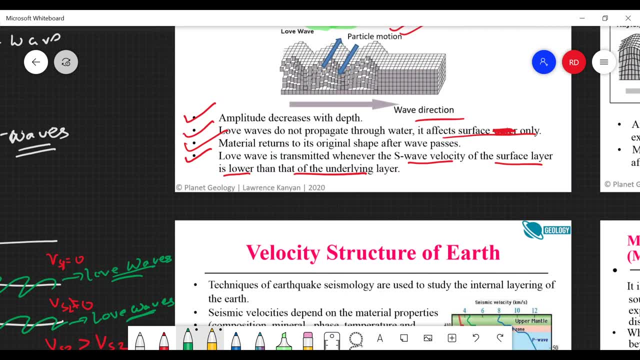 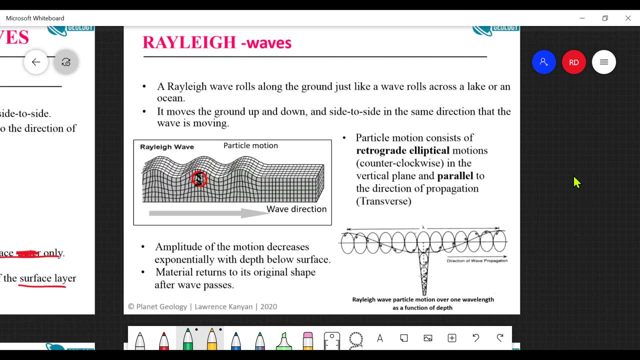 These love waves? Okay, There is no as such ground surface over there, but between the borehole wall and and and the rocks there, you will generate some love waves. Okay, Rayleigh waves, They're like waves that you see on surface of water. 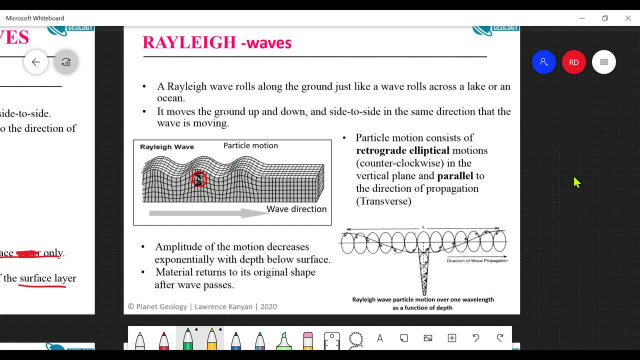 Okay, If you have gone to the beach deeper into the ocean, you see those waves and those are sort of a rolling motion. They are type of a Rayleigh wave. Okay. So these These waves roll on the ground just like waves roll across a lake or an ocean. 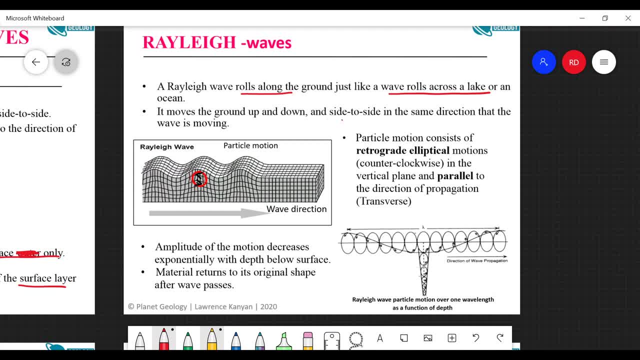 Okay, It moves the ground up and down and from side to side in the same direction that the wave is moving. Okay, So these are more of like an elliptical wave. The motion of the ellipse is retrograde. This is the particle motion. 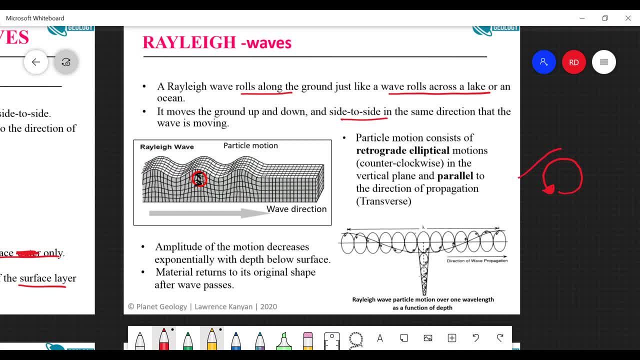 Okay, And, and and. the wave is is basically traveling like this: Okay, And they will die down. They will die down with, with, with like distance from the surface. So you can see here, these, these are type of Rayleigh waves in here. 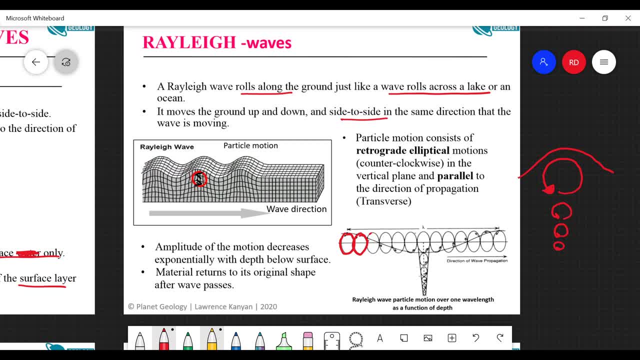 Okay, So here, actually, multiple particle motions. Again, the particle motion is what we call retrograde. Okay, Why? Because if the wave is moving in this direction of propagation, this is direction of propagation. So this is the direction of propagation. 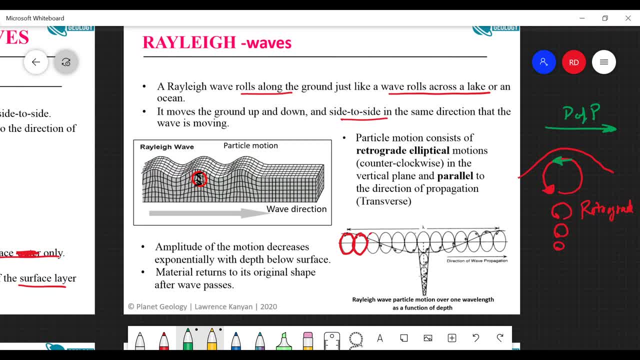 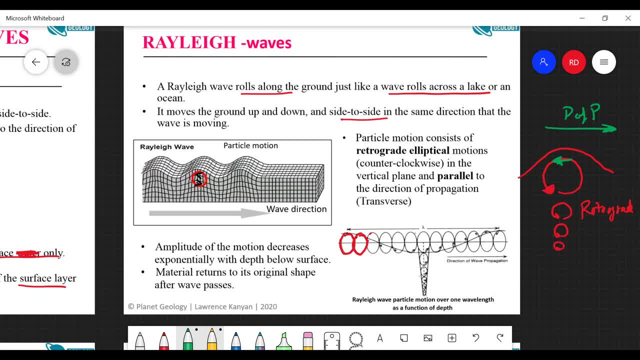 So the direction of propagation, uh is, is what you will scale. The motion is retrograde. That is why the name of this motion is retrograde. elliptical motions, Okay, In the vertical plane and parallel to direction of propagation, Okay. 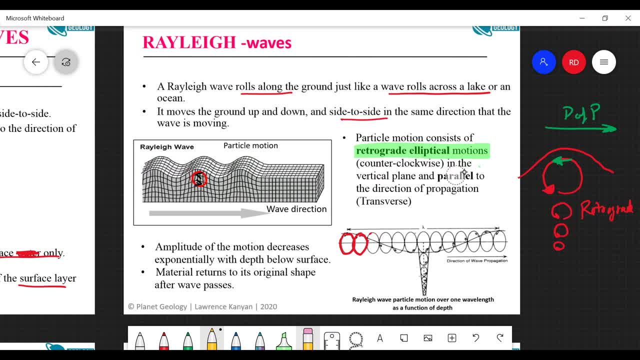 So it shouldn't be like Parallel it, it should really be: on top It is parallel, but here it is vertical, actually perpendicular, Okay, Because then this will not be parallel. I think this is the wrong here. So this, this is counter retrograde elliptical motion overall, because this ellipse is more like this: 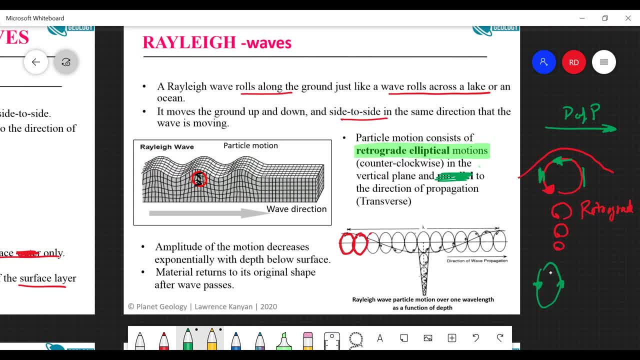 So it's, it's still going up and down, So it's it's sort of like a transverse motion, only because you are, the wave is traveling in this particular direction. Okay, So this is this is how how this, this motion occurs, and the wave that you see here is: is this wave in here? 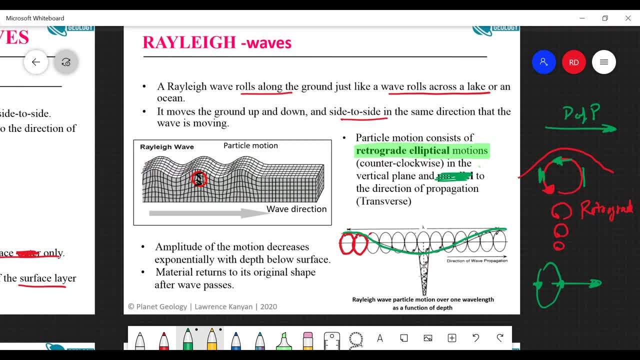 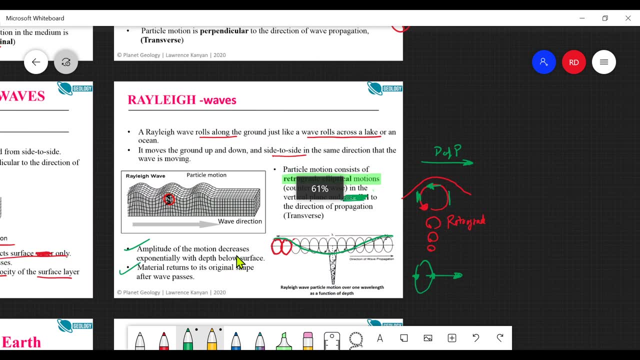 All right. Amplitude of the motion again decreases exponentially with depth and material returns to its original shape after the wave. In general, like for for for normal frequencies, Rayleigh waves are slower than love waves, Okay, And they also have higher amplitude than love waves. 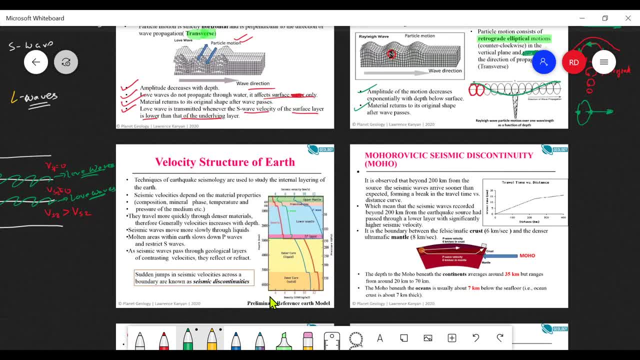 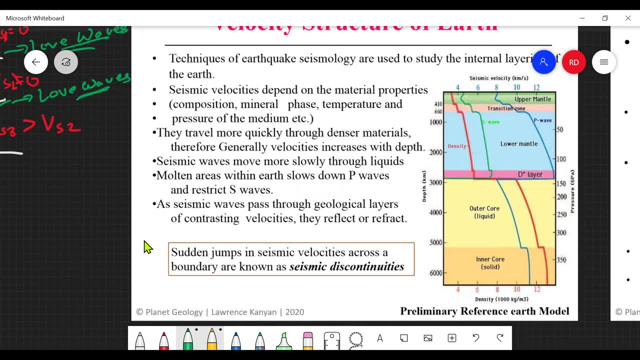 For For normal frequencies that you see, not for very low frequencies it may not be true, but it it is dependent on frequency. but usually you'll see that Rayleigh waves generally are slower than love waves. Any questions? We are, we're done with the, the, the P wave, S wave. 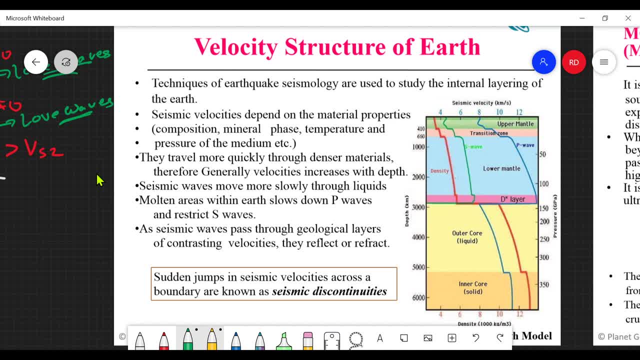 We lost different types of waves. Any any questions? Again, very important. You need to have these notes in your notebooks. This question will be asked in in the civil Services exam. very high chance. There is very high chance of this question being asked. 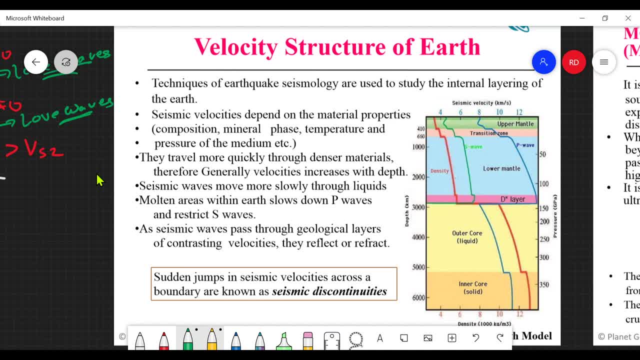 Any questions? So, Chandan, you are asking how to structure your answer relative to types. Okay, So first of all, in your answer, when you're writing, first of all, if, let's say, you just don't start, like, with types of seismic waves, you 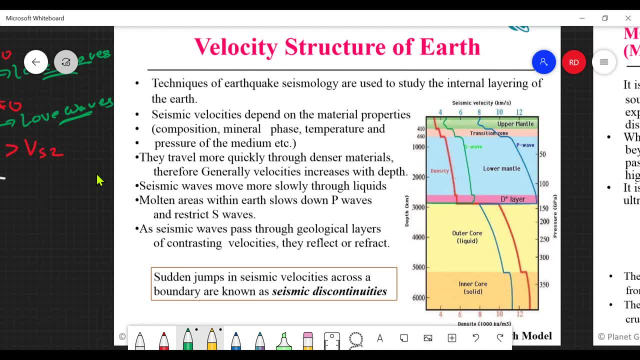 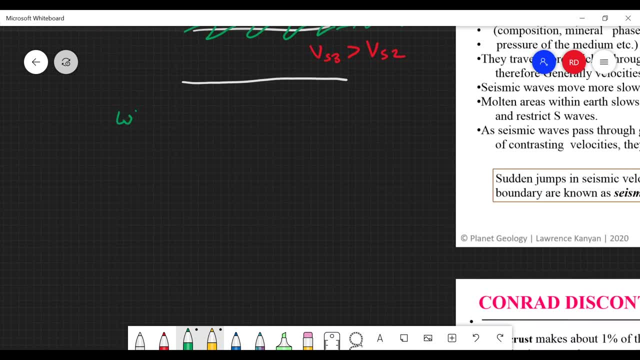 define what seismic waves are. so that is given in the very first slide: What seismic waves are, okay. what? okay, why? okay, what seismic waves are. so why do we actually study seismic waves? why are they important? You have to write first this part, okay, they? 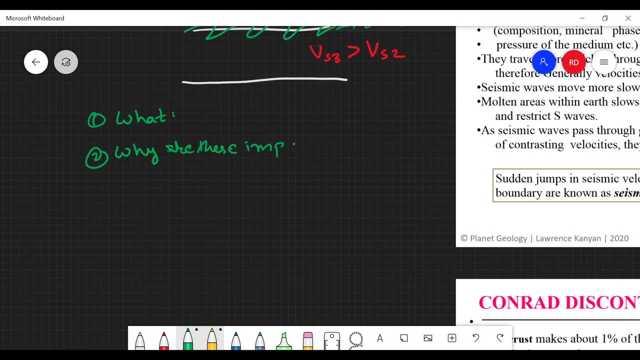 tell us about the internal structure of the earth. so now you are building a little bit story. then you come to third type. you define the types. okay, you define the types. Now again, as I said, it's not always possible to give you the given answer in one question. 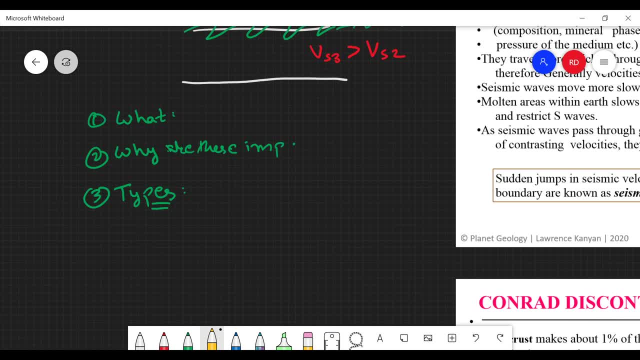 okay, what will come into the subsequent slides? you have to learn to incorporate that also. okay, maybe that part is not given in the P wave, S wave parts itself. for example, when you say these types, P, S, L, R, so you say S waves, for example, importance you. 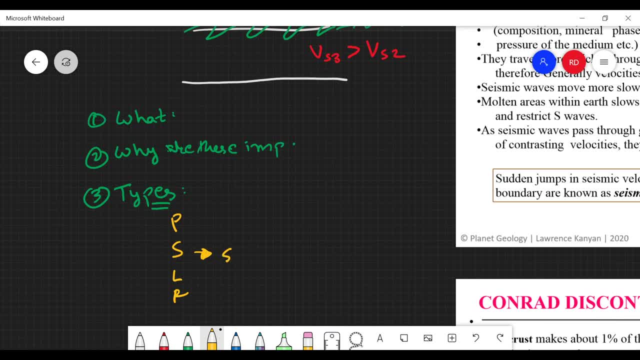 can mention there also. so you will define all these terms. shadow zone concept- maybe they have not asked you itself now, S waves are important Because of this shadow zone. S wave shadow zone. S wave shadow zone tells us about the outer core of the earth and that the outer core is in a liquid state. okay, it tells. 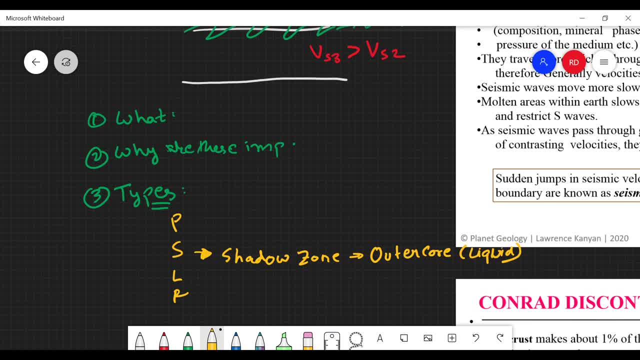 us that this outer core is in a liquid state, so this becomes important in that regard. okay, so you, it's not that whatever material is mentioned here, you just have to write it. now it's not possible, for example, for me: if you have a, if you have a, if you have. 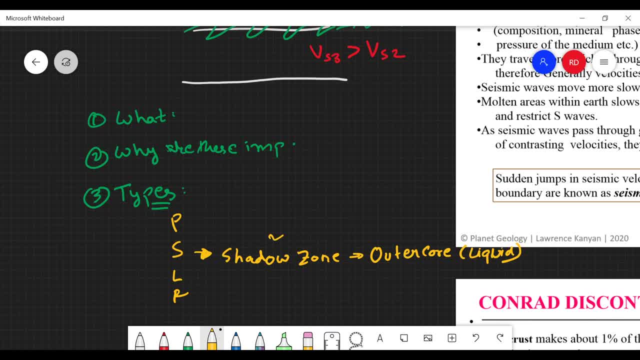 a, if I write shadow zone, then questions will come: what is shadow zone? and all that is separate topic. but you, you can write about those particular things, okay. so these, these are again important. so you write about types of of these, different types of. 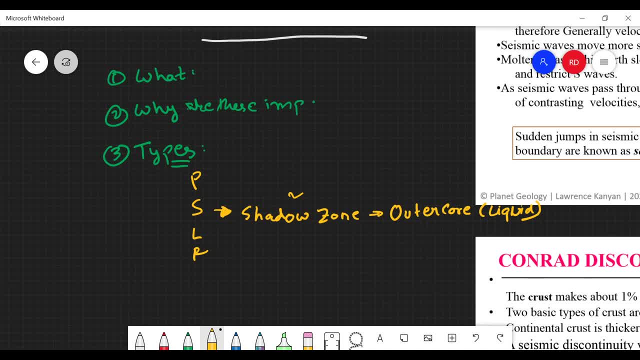 waves, or okay. so so then you, you have defined all, all these types, okay, and then in, in, in fourth, if, if you, if you have time, this is not mandatory, you can conclude with with a one line: but again, this is, this is not mandatory, you can, you, can you. 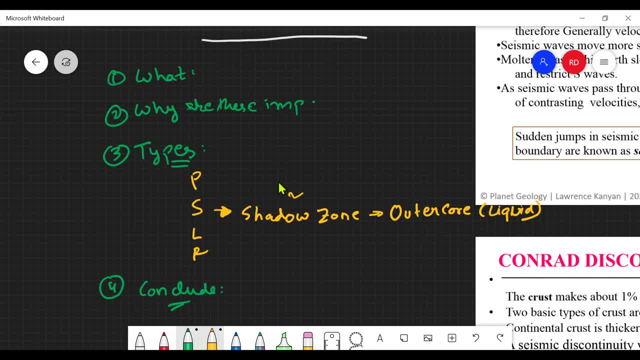 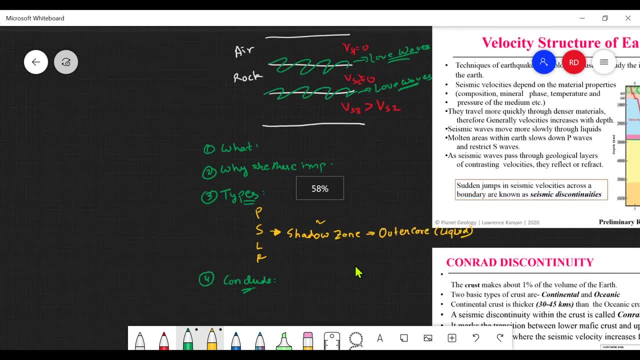 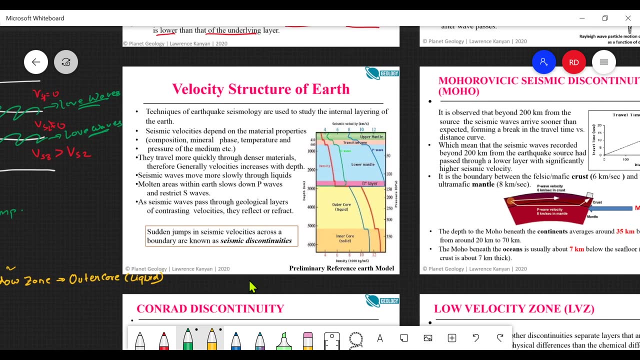 can write: okay, so these different types of waves are there and then their travelling behaviour can tell us about the internal structure of the earth. okay, so this is how you will write your answer, okay? usually there is no direct answer to those which are more destructive. 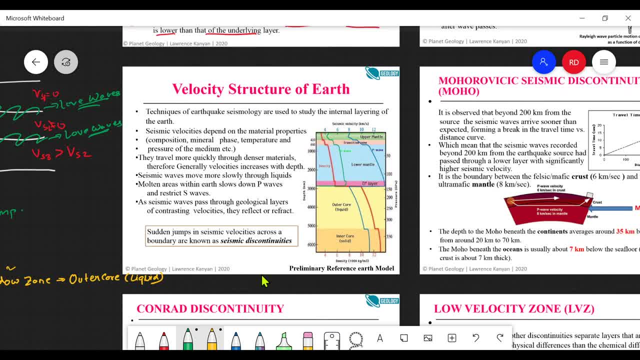 L waves or S waves, a lot will depend on the structure that is there on the ground. okay, so usually L waves and S waves we usually you will see- it is mentioned that surface are- are pretty destructive. okay, a lot will depend on the structure as well how that. 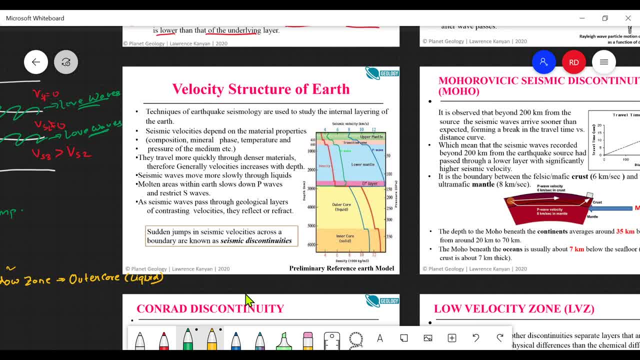 structure interacts with, with those surface waves. okay, based on on amplitude, again, it's it's. it's not true. for it, it depends on frequency also, how, how these L waves and R waves will behave. okay, for very low frequencies, it's, it's slightly different. 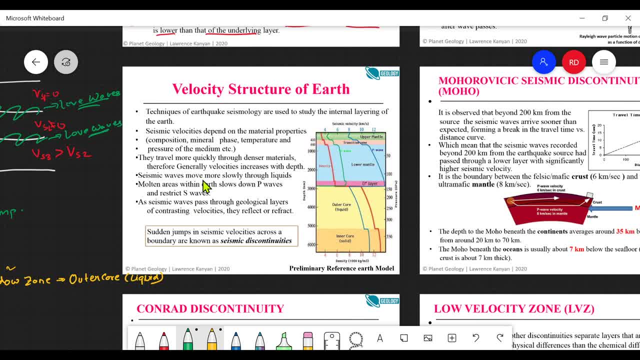 relation, but usually we just say that surface waves are more destructive than body waves. all right, okay, so in the we will take, we will take a very short break here. okay, so so that.